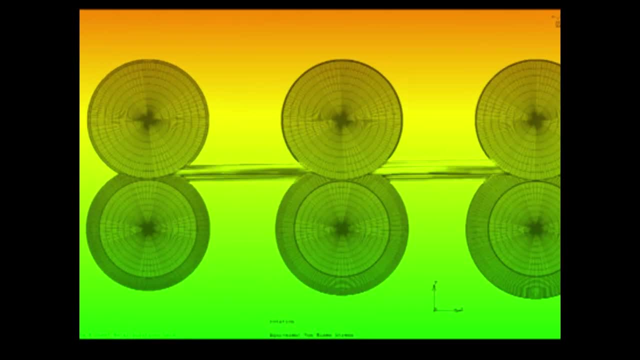 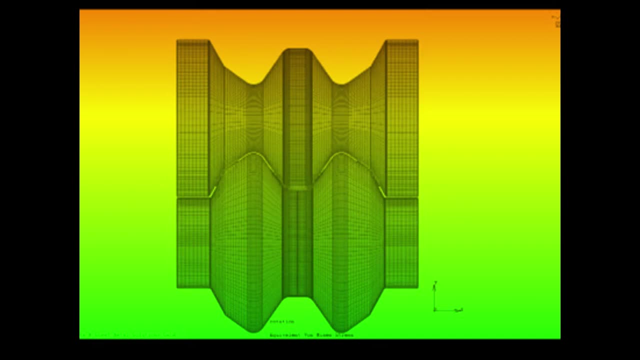 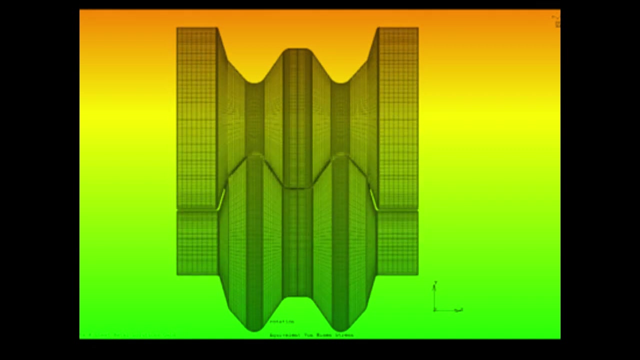 to give the material a good straight square start into the rolls where the forming takes place. Next in the line is the role-forming mill itself, And we've drawn here schematically a mill with 16 passes. Well, quite honestly, there's anything from only a couple of passes up to 30 and more passes in some role-forming machines. 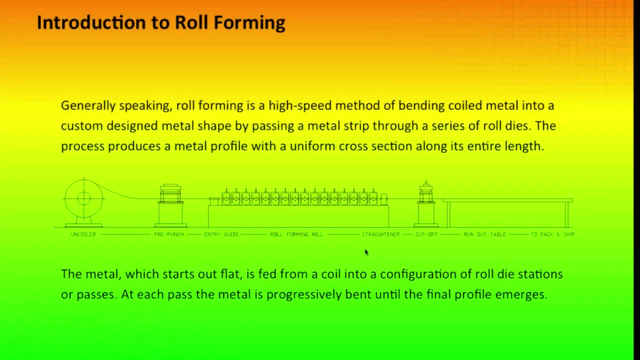 This is where the forming of the actual profile takes place in the mill. Then, at the exit end of the mill, there is a straightening device, And here's where we tweak the part a little bit. By this point it's at its finished and final shape. 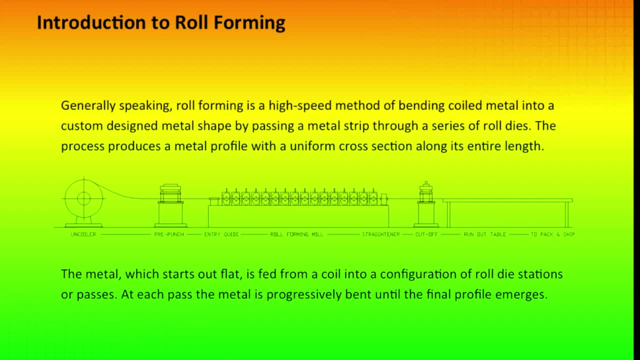 But there may be some adjustments needed to compensate for a slight twist, camber, bow, et cetera. The next piece of equipment- A typical role-forming line, generally speaking, is a cut-off press where we would cut off the part to length. 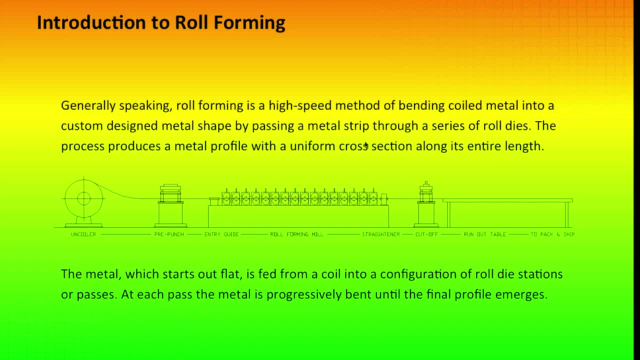 There could also be a post-punching press between the mill and the cut-off press, But in this case we didn't draw it that way. The part is cut to length and then it is put on a run-off table or a run-off bar. 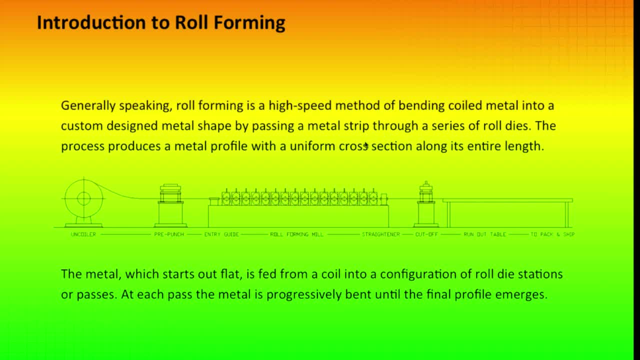 where it's made ready to either be packed into shipping containers to go out to the customer or perhaps pre-packed. Then it's put onto a cart and moved to another place in the facility for additional secondary operations. Sorry to interject but I just want to know. can you see the screen now? 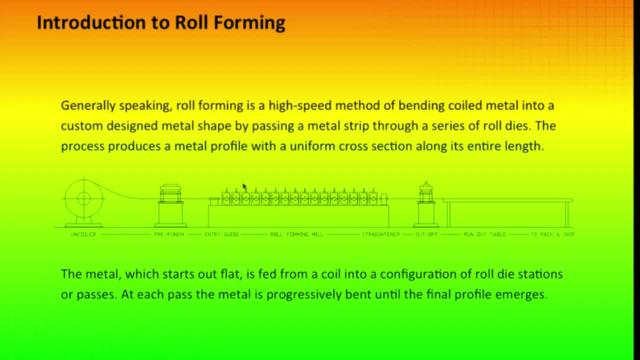 No, we can't, Okay. Well, I just heard from one of our attendees that they can see the screen, So there just might be something wrong with your screen. I will just say to our attendees: if you're having problems, please use your question box right now to let me know. 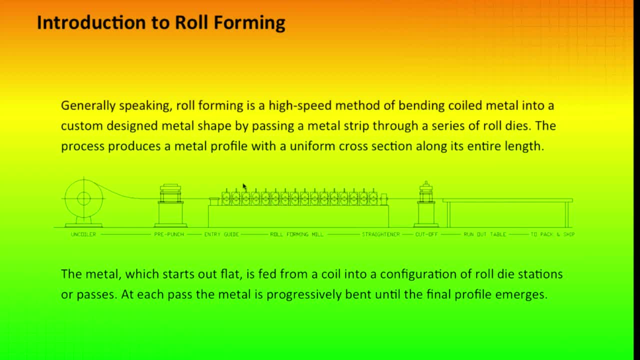 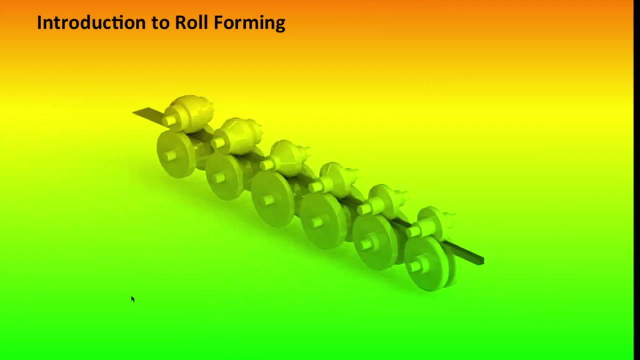 But, as far as I can tell, the screen is showing and I'm told that people can see it just fine, So we'll continue, Okay, All right, So let's go on from here. Let's go to the next slide, Alan, which will show a set of roll tools- roller dyes. 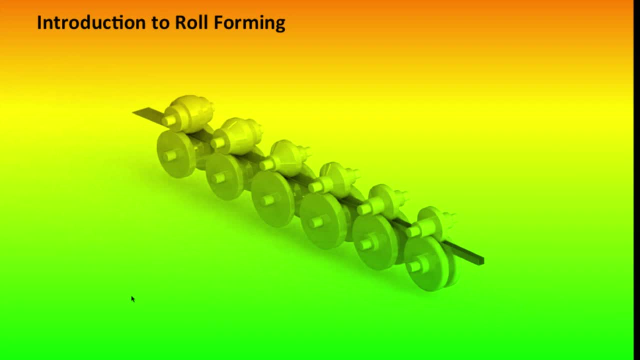 What you see here pictured is a model of a typical set of roll form tooling. You'll often hear roll formers speak of passes, of tools, and that's how we refer to ECC. Okay, We refer to each set of top and bottom or male and female rolls. 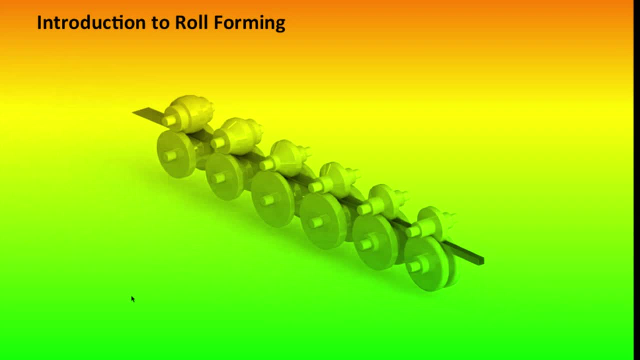 And if you count them here, in this model there are actually six passes. They're not shown in the mill but they're showing as though they were set up in the mill. the light blue spindles indicating the machine shafts At the top left. the stock from the uncoiler would enter into the mill. 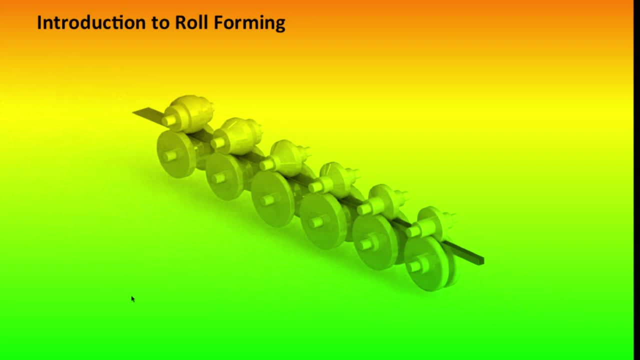 The first pass as a flat strip and then progressively formed in each pass, going from pass one at the top left to pass six, in this case to the bottom right where you'll see the final channel shape, in this case a simple U-channel. 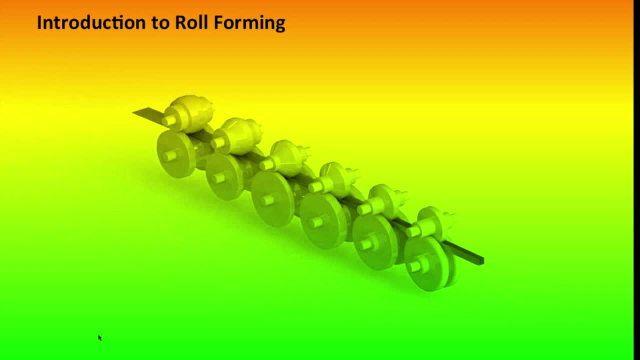 exiting the last pass of the mill. Just a side note here. This is really just a representation of what you might expect to see. A light gauge U-channel or a light gauge part, short legs, very simple, might not even take six forming paths. 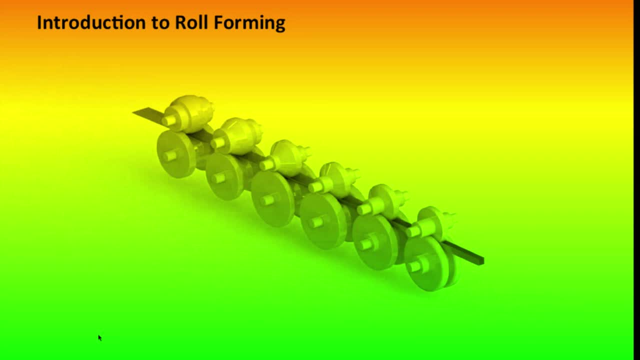 On the other hand, you might require many more passes if the shape is complex or it's a very deep channel. So just keep in mind this is just representative of what roll tooling would look like set up in the mill. And Alan, let's go on to the next slide. 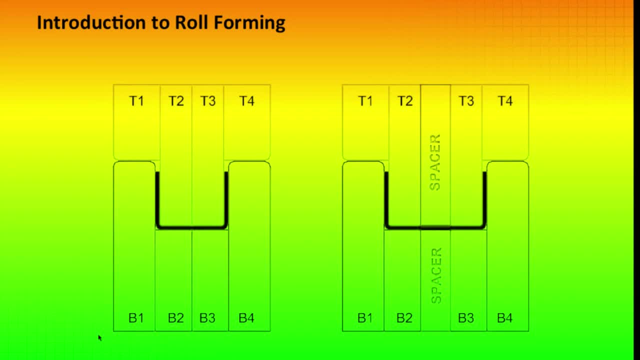 What we want to do here is take a look at what would be representative of a single pass of roll form tooling. Now let's focus on the section over at the upper left where it says: there's a green outline there at the top of the rolls- T1,, T2,, T3, T4,. 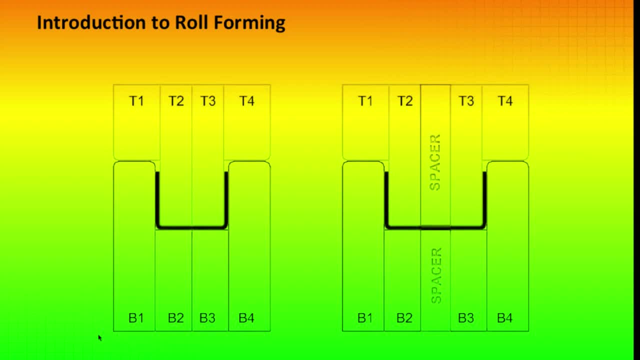 representing the top roll or roll set, And then B1 through B4 in blue represents the bottom, which is the bottom set of that pass. So what we're showing here is like an end view or a cross-section view, something similar to what a tooling engineer would design for the building of these rolls. 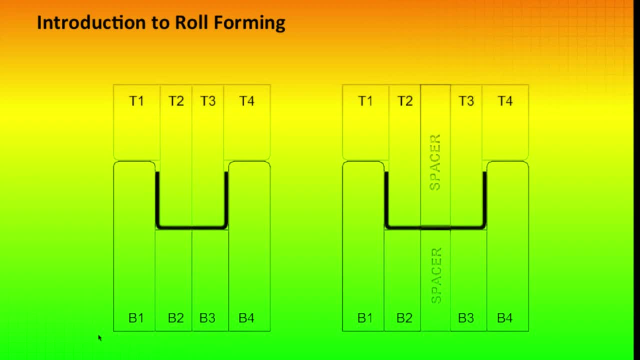 of course, without dimensions, And you'll notice that the rolls are segmented or split. Sometimes we call them slices, And we have really a couple of basic reasons for doing that. First of all, segmented rolls are much easier for manufacturing purposes, Rather than cutting the whole top or the whole bottom out of a single billet of some tool steel. 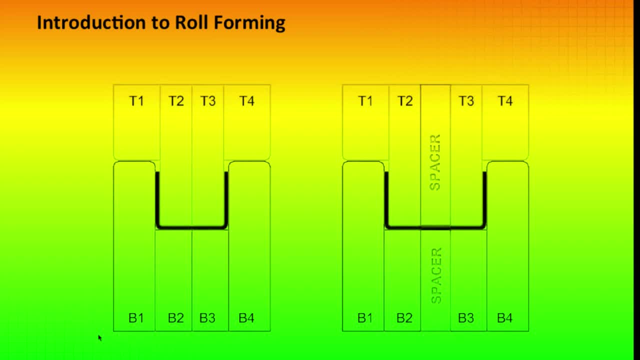 we cut slices that are each closer to the finished size, so we waste less material. And, being segmented, it's also easier for handling for the operators When they're going to put these in and out of a machine. the individual segments, of course. 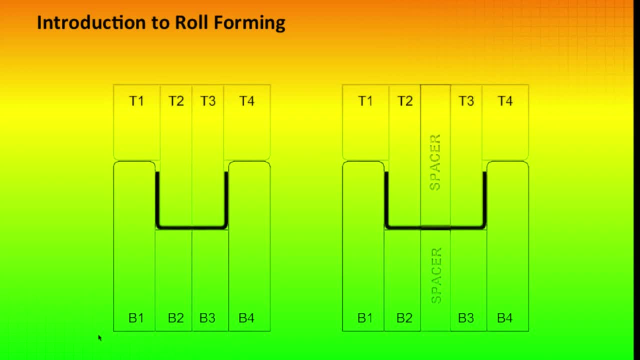 are lighter than if you had the whole top roll to put on the shaft as a single piece, and the bottom too, of course. The other reason that we segment these is because it gives us a chance to use these as a universal channel set. 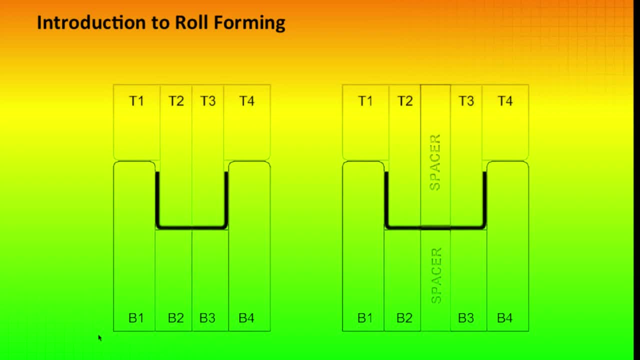 For instance, if you look over at the right-hand side of the same illustration, there are two spacers marked in red. What that means is we could take the same tool set that's shown in the left, add some spacers and use the same basic set of tools to make a wider channel. 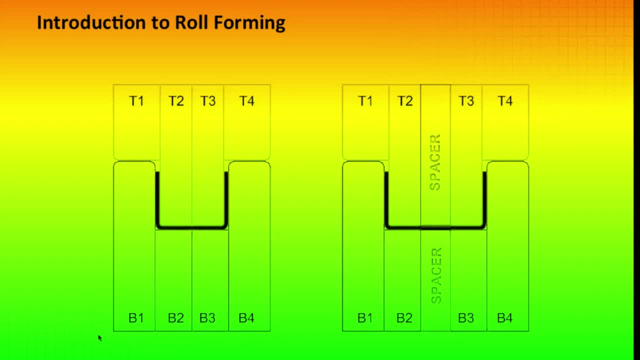 Also possible. you could change gauges many times in these same rolls because they're segmented and you make the compensation for the various material thicknesses by use of shims and or spacers. So the universal channel approach is really good for a simple product like a U-channel. 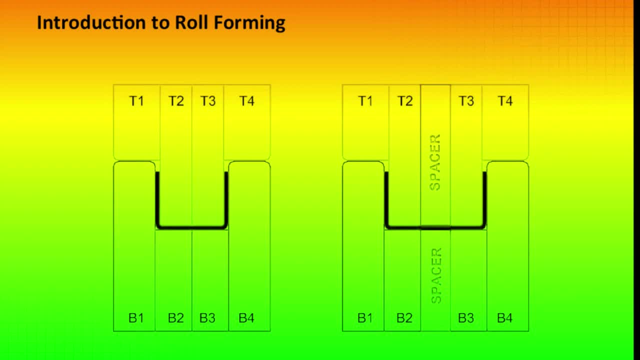 and we also have universal angle dies so you can have a variety of angles, different leg lengths on a simple 90-degree bend, And you can do similar things with hat channels, struts, Cs, that kind of thing. It really saves an awful lot of money for the customer. 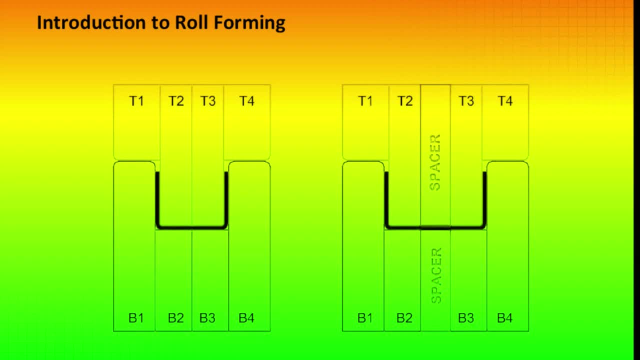 because you can take advantage of an existing set of tools and then perhaps, rather than buying a full tool set, you can use our existing tools and just pay for a few spacers. It's a huge savings in tooling cost. The next slide. let's look at the next one. 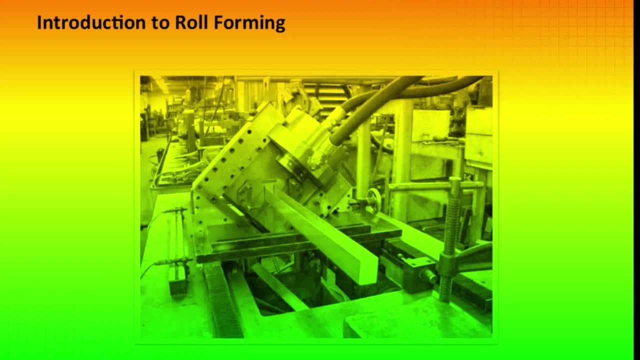 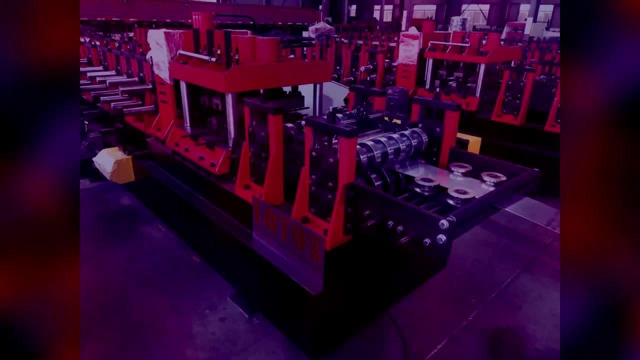 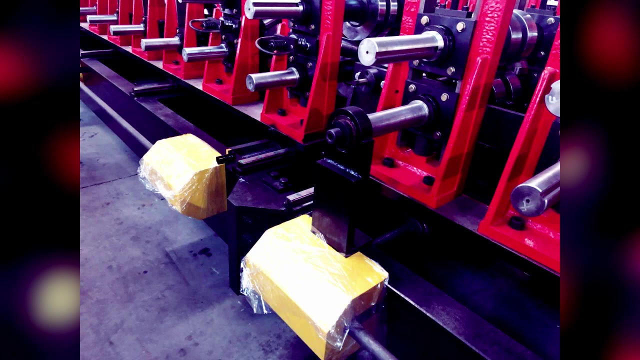 It shows the final operation in the line and that is the cutoff press. We're looking at the exit end of a hydraulic cutoff press that we use on a line very similar to what we've indicated here in this schematic. It's a proprietary design, uses a servo-driven, slugless cutoff. 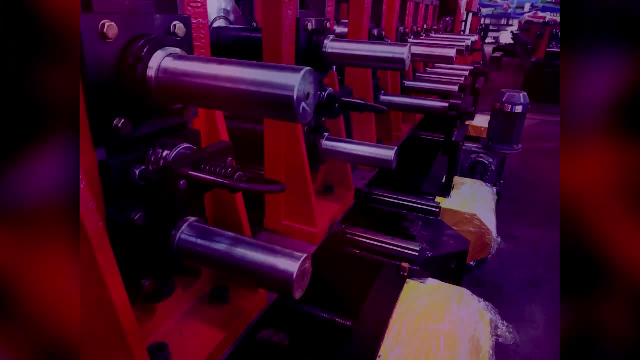 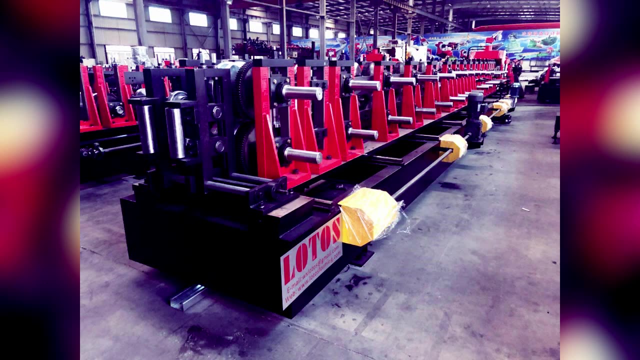 Basically for an open shape, we can use a couple of steel plates that have a wire EDM through them that matches the profile, with minimal clearance around it, so that when the die fires, the press fires, there's a shearing action that takes place. 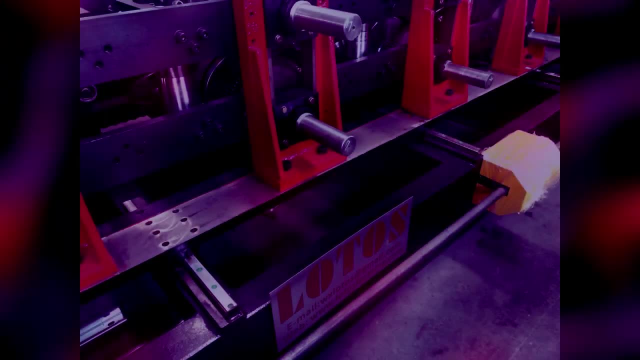 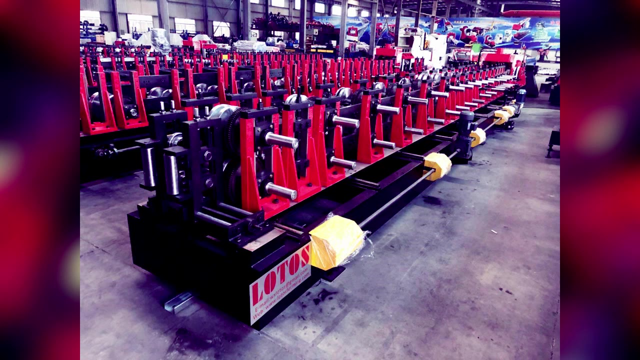 and it removes or cuts to length the finished piece from the roll form product. cuts it to length and produces no slug, so there's no waste and minimal burr, which is always a good thing. It's very intelligent, very efficient. 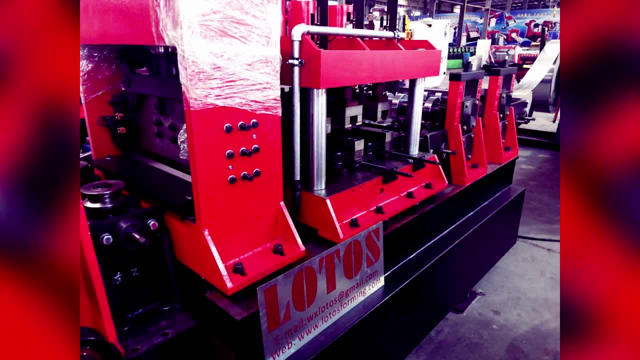 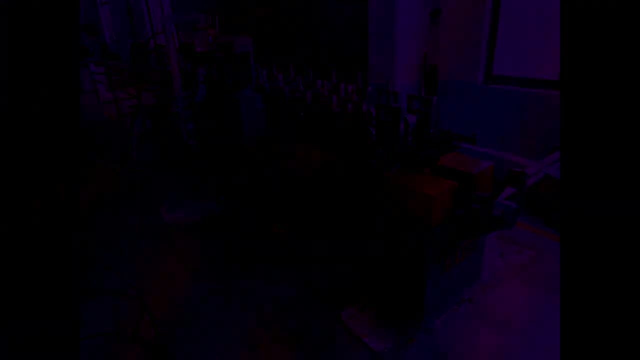 The die sits at its home position until it's signaled by the controls to go out at line speed to the correct position and then very accurately cut off the product to the correct length, and then it'll come back to the home position ready for its next cut. 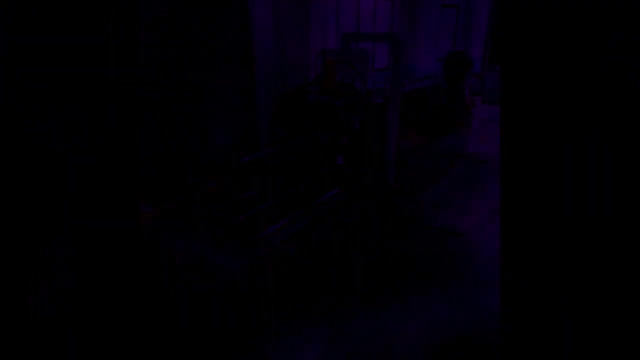 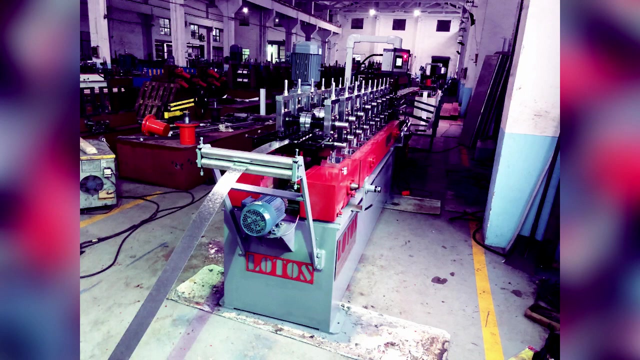 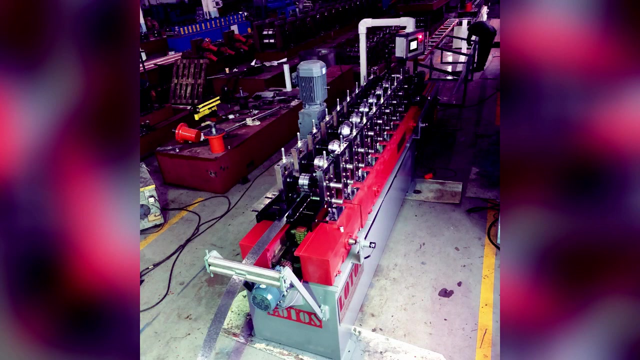 So think about how efficient that really makes it. Other than having to load coils or perhaps move loads of finished product out of the way, the operator really never has to shut the machine down. It's a continuous operation. flying cutoff parts go on the load. 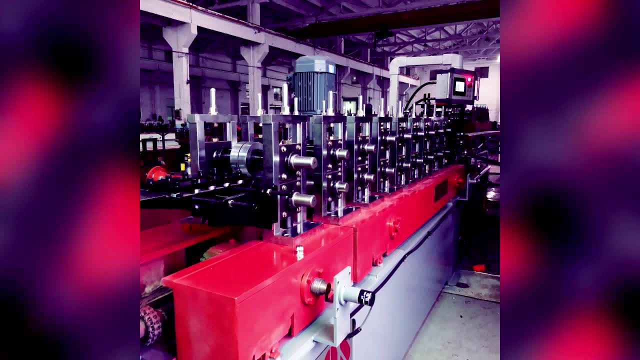 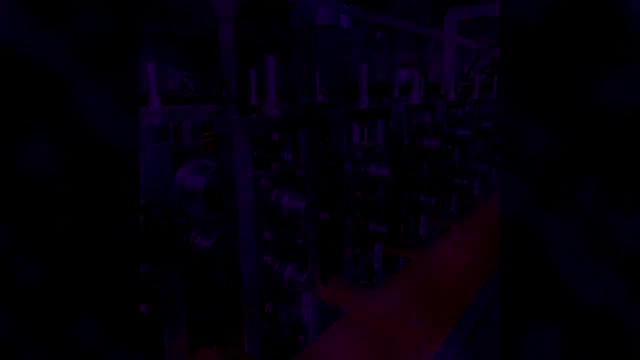 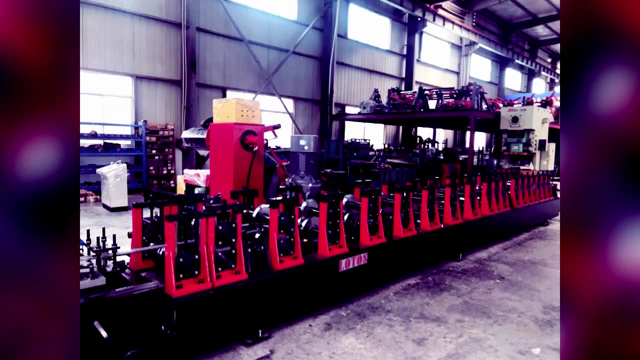 and ready to just continue with its production. So that was a basic description of the introduction to roll forming, based around a very typical roll forming line. What we drew there in the schematic and the description we'd given you certainly is not all inclusive. Not every roll forming line looks like what we do. 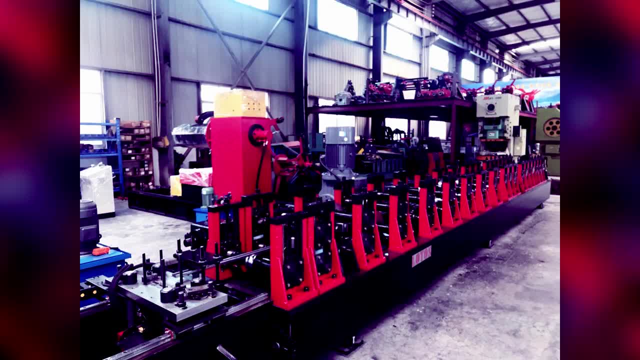 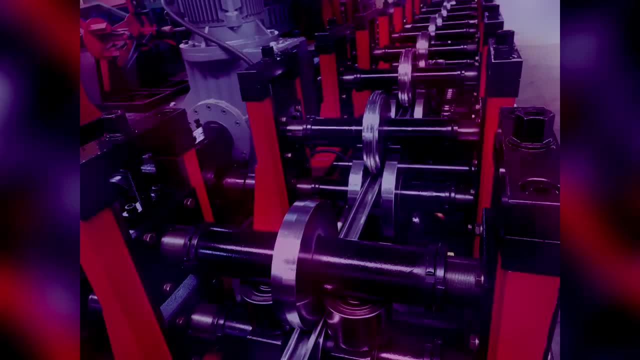 Not every roll forming line looks like what we've demonstrated here, But this is typical. You could have more presses either before the roll former or after. Some people have presses in the middle of the roll former, So there's almost an endless amount of variation in how the line can be set up. 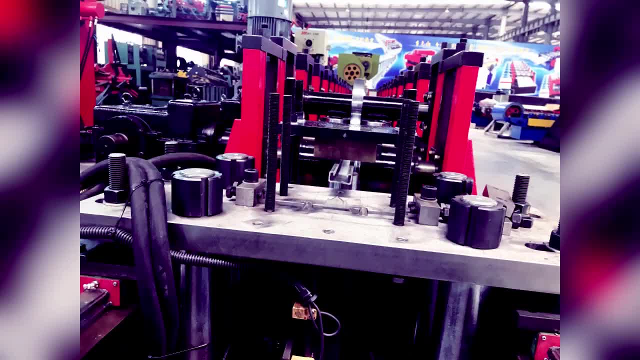 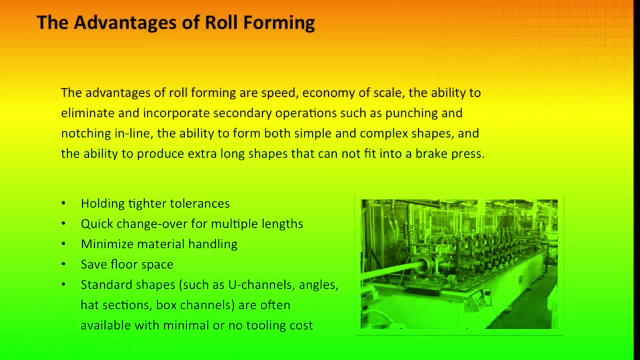 But this gives you, I think, a good idea of how the process works. So, moving on here, our next subject we want to cover is the advantages of roll forming. If you turn over, I'm on the next slide there, Alan. 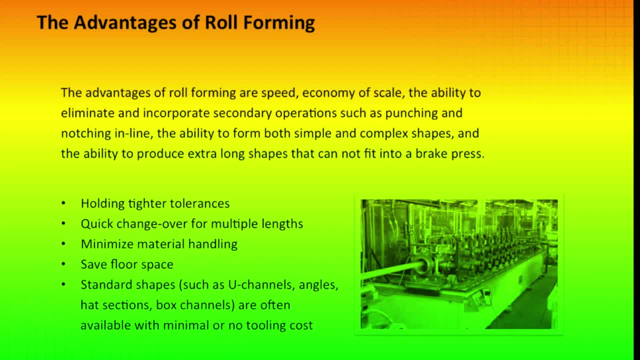 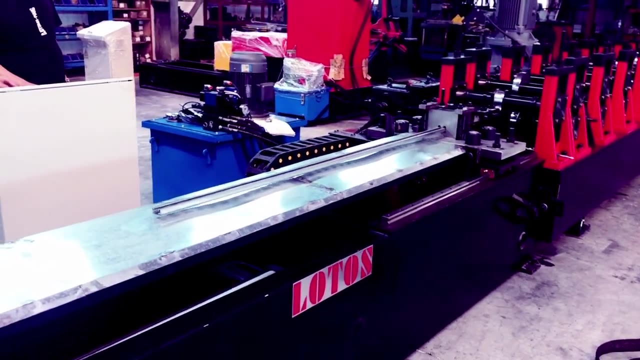 Yep, All right. So the paragraph says here that it's advantages are speed. We can incorporate secondary operations in line, We can do very complex shapes as well as simple ones and make extra long parts that you probably couldn't produce in a break. 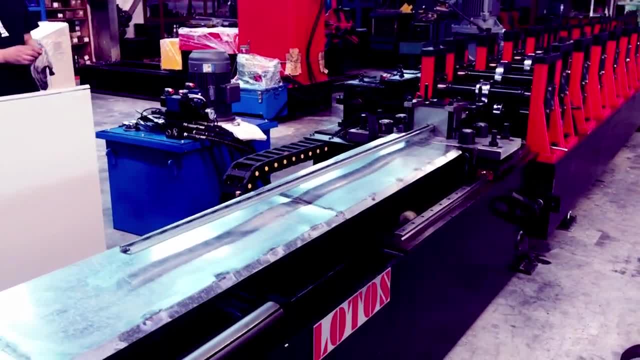 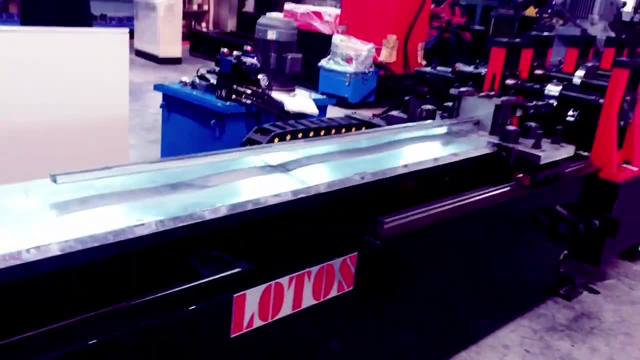 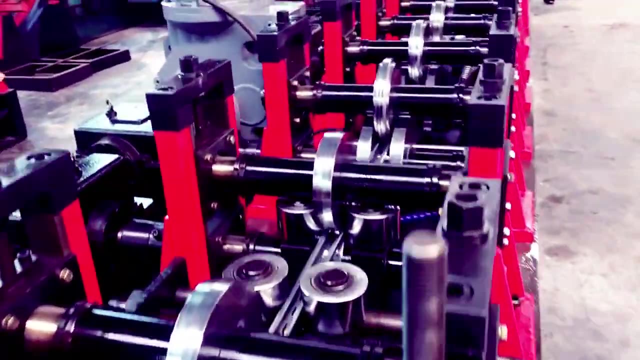 So then down along the bullet points there, holding tighter tolerances, Typically roll form product. because we have so many opportunities to control dimensions in the toolset, we can control dimensions, cross-sectional dimensions, much more closely than other metal forming processes, for instance a break. 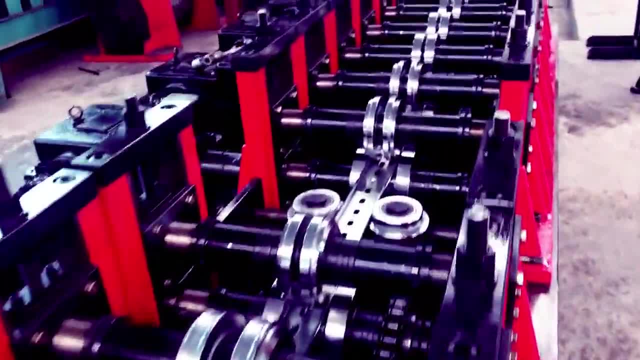 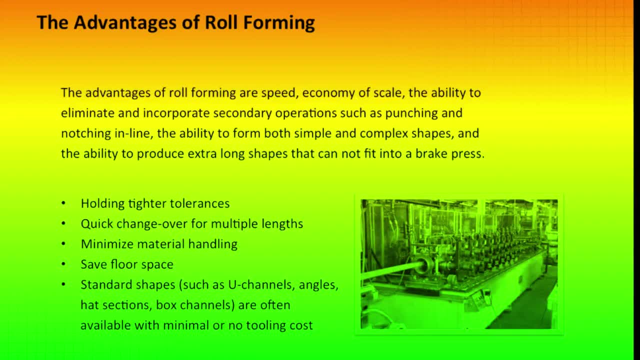 When we're changing part lengths. it's really something that we can do on the fly. Quite often we can just put a new length into our controller for the line and go from 48-inch parts, let's say, to 60-inch length parts. 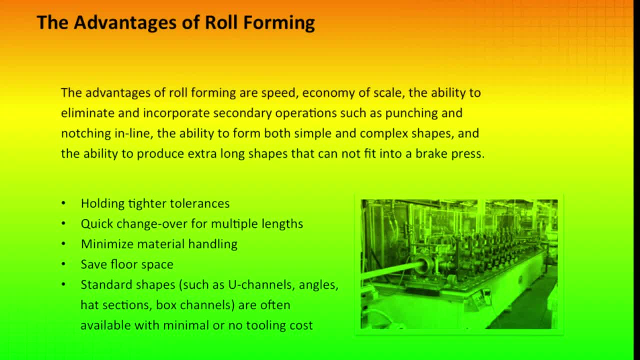 Without moving a physical mechanical stop or anything like that, And because we're running a continuous production from coil and cutting it to length. Material handling and saving on floor space- they both kind of go hand in hand, If you think about the line that we just described. 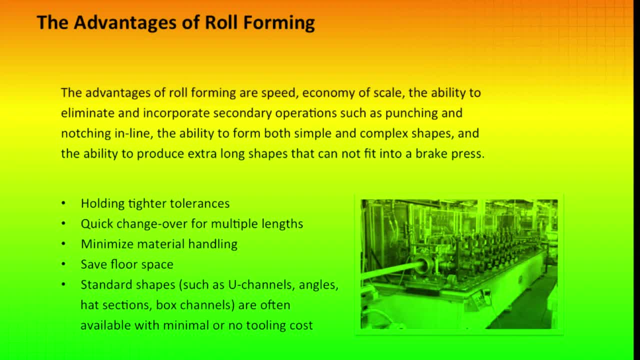 a coil of steel goes on the entry end of the mill. Operations take place in the pre-punch, perhaps forming through the mill, perhaps additional operations in a post-punch and or the cut-off And out the end comes a part that is a net part. 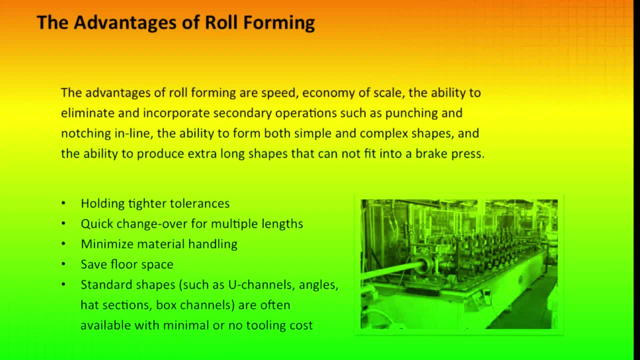 basically finished with all its features included, generally speaking. So we don't have blanks sitting around on skids or trucks. We don't have partially finished pieces that have had notches or a bend and waiting for the second bend From start to finish, whatever amount of floor space that machine takes up and the load. 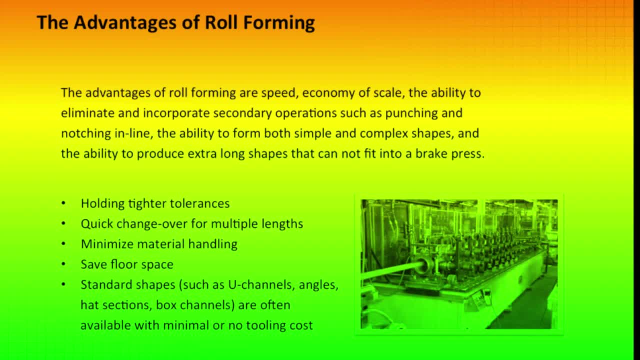 and then the part is moved off to shipping or perhaps to a secondary operation. So we save floor space and handle much less product in our building. The last point there, which we've touched on earlier: standard shapes such as U-channels, angles, hats and box, or C-channels. 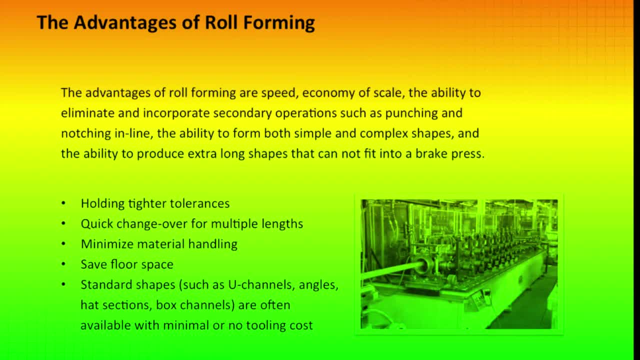 are often available with minimal or no tooling cost, And that's for the reasons we already described Many times. there are standard or universal channel and angle sets that will fit the bill for what you're looking for. So in those cases, maybe just spacers, maybe just some cut-off tooling. 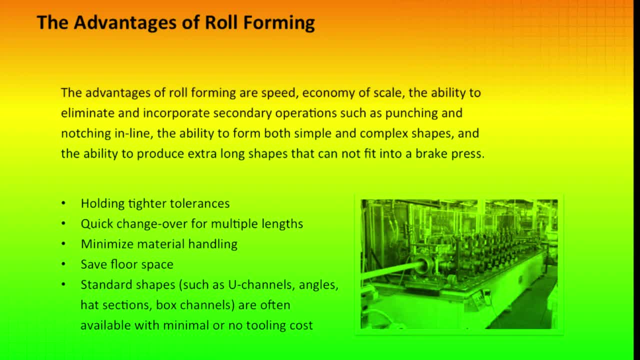 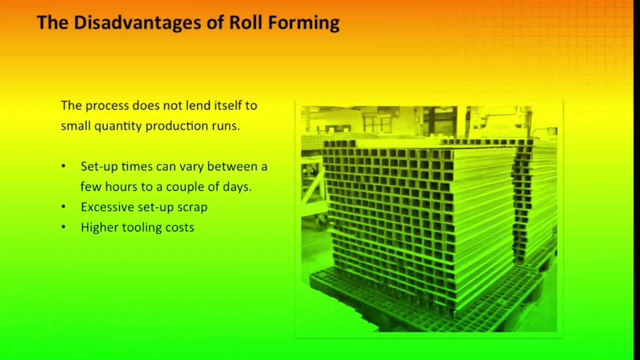 certainly a lot less expensive from a tooling standpoint. a brand-new set of tools Then on our next page. certainly like any process, there are some disadvantages, And probably the single largest one with roll forming: it just doesn't lend itself very well. 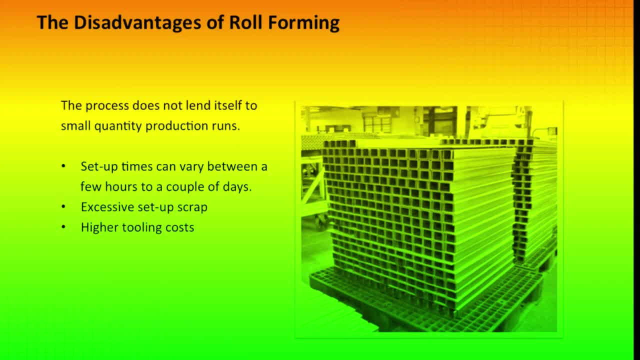 It's a very small production quantities When you think about what goes on here at times. for very simple shapes we can set up a machine in a few short hours, But more complex shapes you may have a day or even two days at times into a setup. 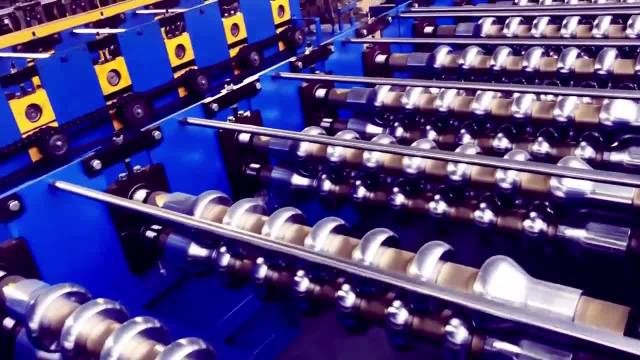 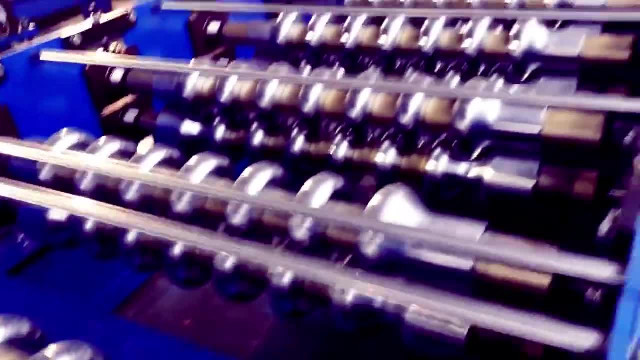 So if the production quantity is very small, all that setup time, along with any setup scrap that's generated to perfect the part during the setup, has to be amortized. All the cost then has to be amortized across a small production quantity. 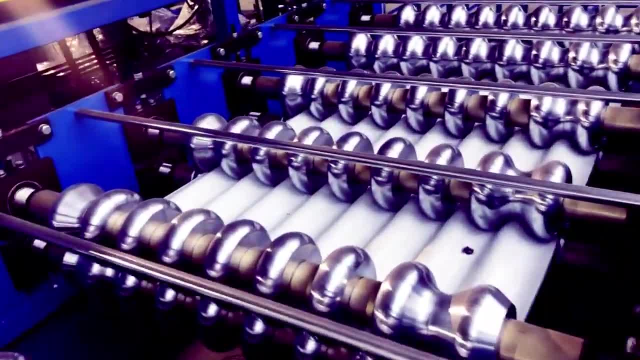 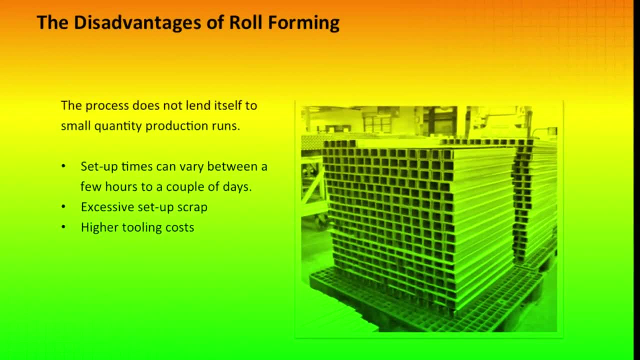 which can drive the per-piece price up. The other thing that's a factor here is potentially higher tooling costs. For a custom shape. that could mean an entirely new set of tools, which could be expensive. On the other hand, many times when more conventional forming and fabricating methods are used, 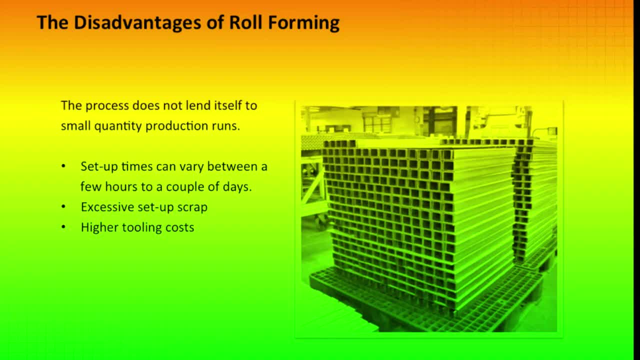 there are multiple dies and multiple tools that have to be built, And each one in its own press and each one in its own operation. With roll forming, we can quite often incorporate a number of features in our pre-punch operations, either by gagging actuating features in and out of the die as needed. 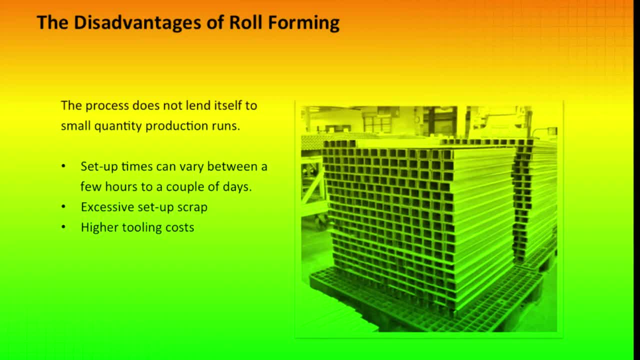 In some cases we have multiple stations in a single die that are individually activated by hydraulic cylinders. So higher tooling costs- not strictly true, but at times it is. So that's one thing that's important. Another thing that would have to be taken into account: 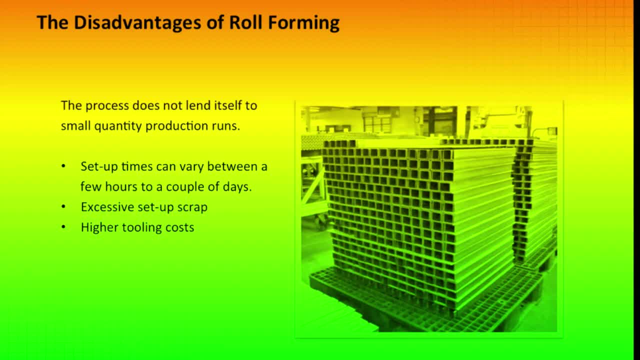 Yes, when you were talking about the quantity, Mike, as far as roll forming, I'd say rule of thumb is about a mile or about 5,000 feet of product. If you have less than that, then you probably should look at conventional. 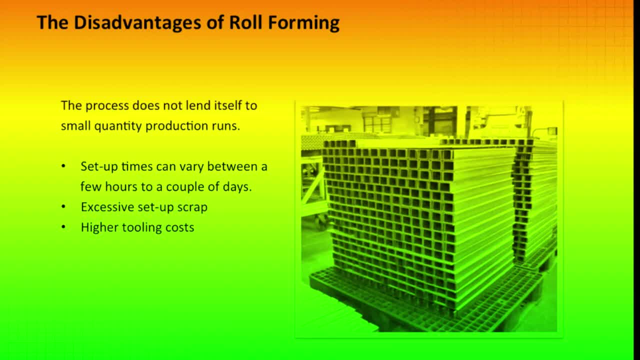 your shear punch and bend operations. When you start to exceed the 5,000-foot level, then you should take a serious look at roll forming, because it does become more economical And, of course, as your quantity, the amount of footage you run through the roll forming line, goes up. 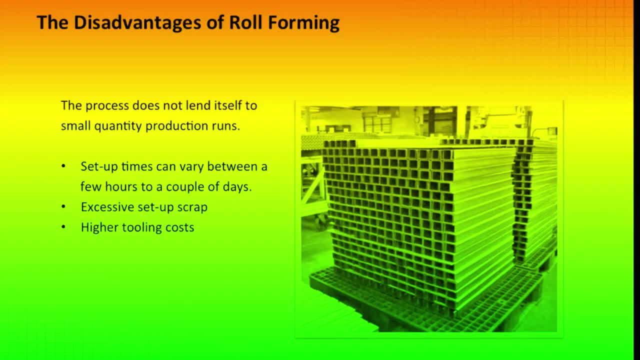 your individual piece price goes down, At some point it will level off, but you'll see a big difference between, say, 5,000 feet and 10,000 feet. But as you get to 15 and 20, your price will start to level off. 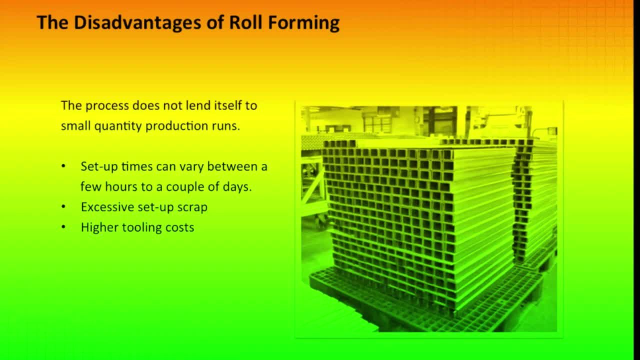 Yeah, that's a good point. One way we've worked around that, and still do, is to take a blanket order for future production requirements. You know Pat mentioned 5,000 feet. Well, if your production requirements for any given time are, say, half of that, 2,500 feet, 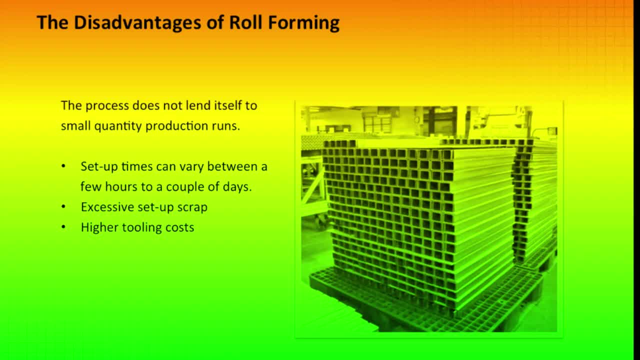 but you still feel that you'd like to take advantage of roll forming. for whatever reason, what quite often we'll do is take a blanket order for future production requirements so that we can, on a single setup, make sure that we have a good production volume would be. 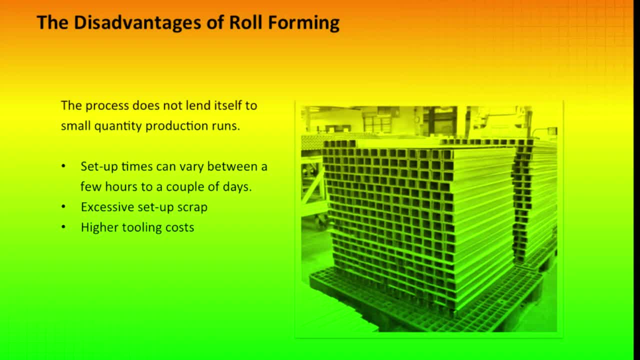 We could run it all at once and that you know. as long as we have an agreement and we know what the dates are, quite often we're able to work that sort of thing out, So don't let that be a showstopper. 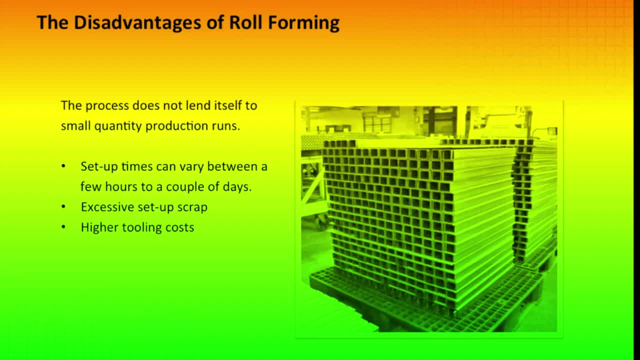 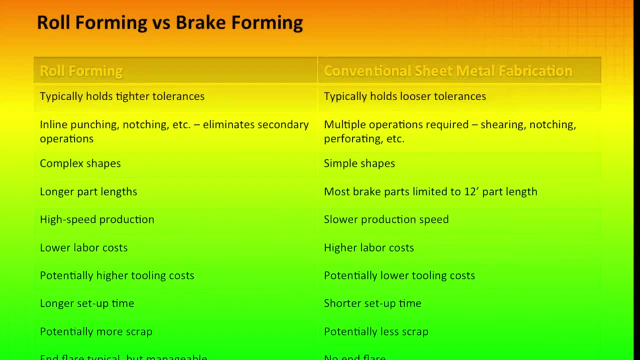 And of course there are times that certain products just can't be produced economically other than by roll forming. So the good thing is just let us take a look at it and see where we can help you with that. So that's kind of the whole inventory when it makes sense. 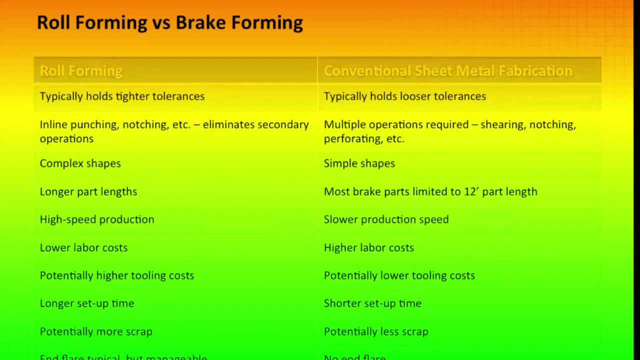 All right, Let's go on to our next page. We've kind of talked about many of these things, but here's kind of a head-to-head, apples-to-apples summary of the pros and cons: roll forming versus conventional metal fabrication. 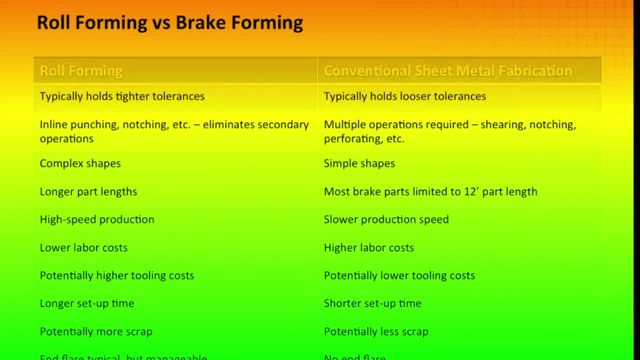 which would include break forming and all the shear, punch et cetera. As we said, roll forming typically wins out when it comes to tolerances. We just seem to have more control over the product than roll forming does. generally speaking, In the roll forming process, as we said, we can include inline punching, notching. 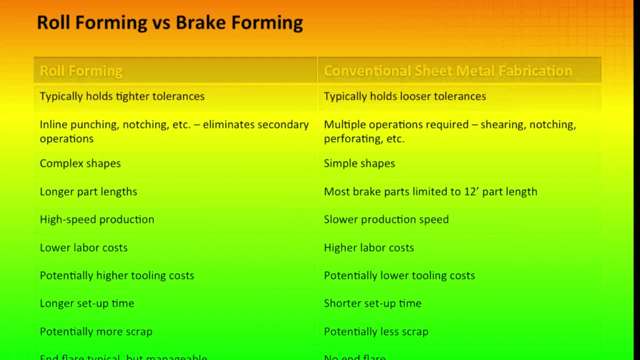 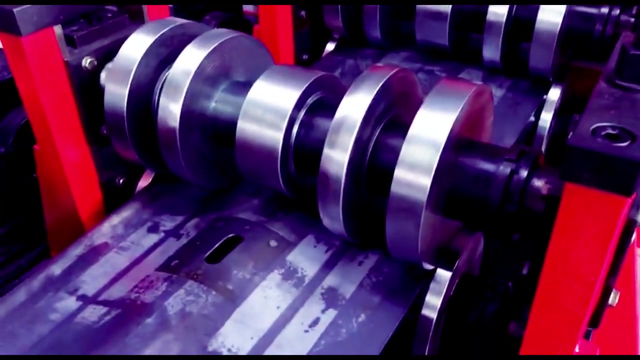 eliminating secondary operations that other fabrication methods would have to use as a separate operation. to include Roll forming, can produce complex and even very complex shapes, whereas more conventional forming is generally simpler shapes: Length of part itself. I've seen parts roll form for rail cars that are in excess of 80 feet long. 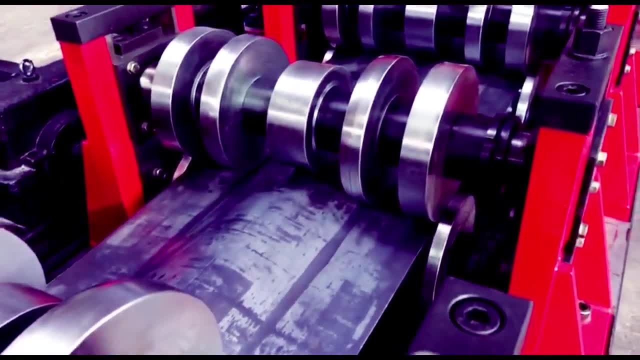 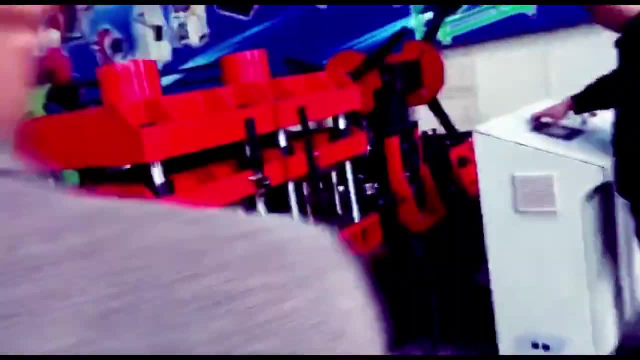 That's not typical but it's possible. You're probably never going to see that on a break, very often limited to the size of the break- 10- or 12-foot break, perhaps a 20-footer at times, But roll forming because it's a continuous forming process. 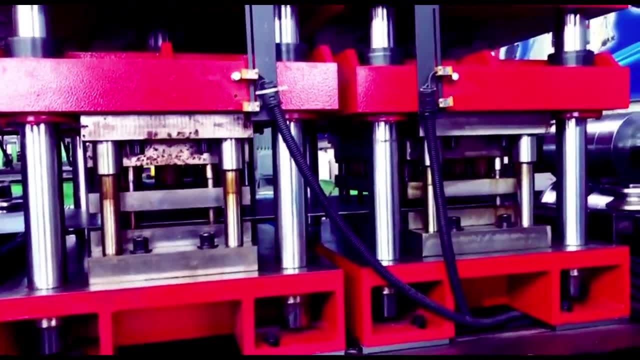 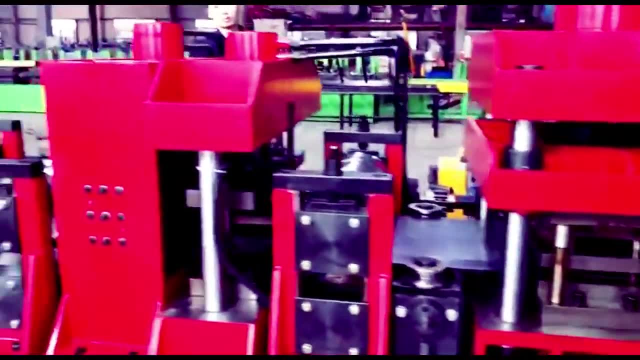 we can cut it off to the length you require And then the only factor that will impact that is material handling and trucking issues. But long parts are certainly an advantage of the roll forming process: High-speed production. once we turn the machine on they run pretty fast. 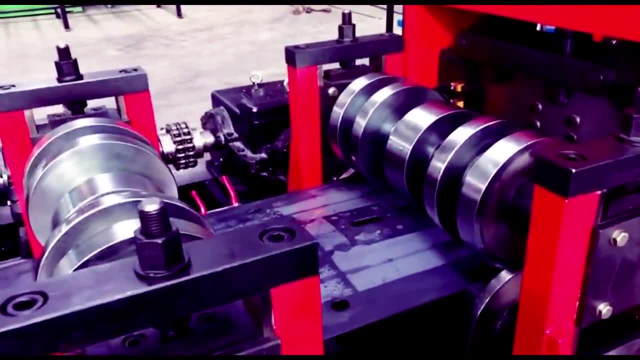 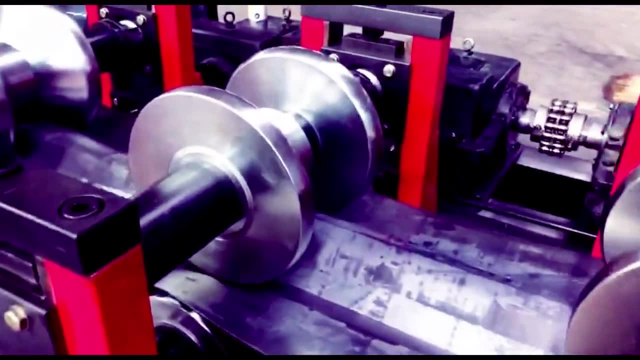 and you really gain some advantage there, especially versus the slower speed of a human being making each bend on a break, along with all the other operations that go into that part. So what that does is result in lower labor costs per part for roll forming. 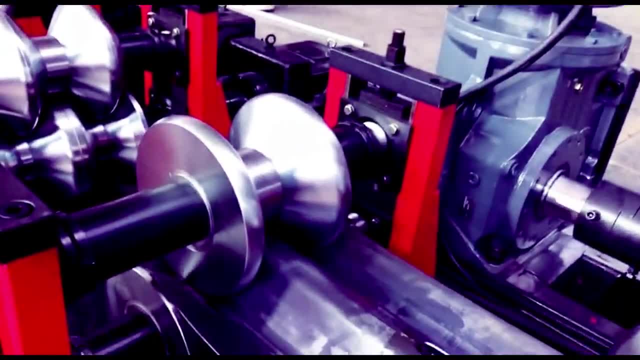 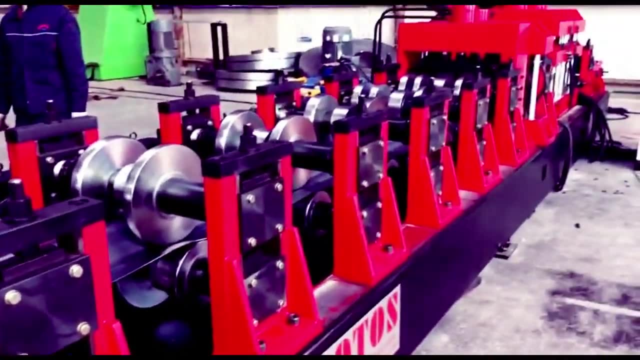 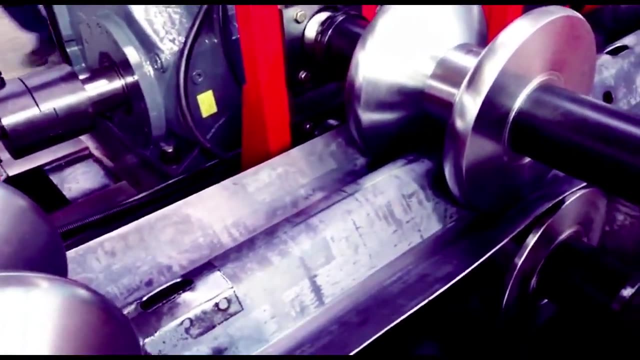 which is an advantage there. One of the disadvantages we mentioned was potentially higher tooling costs for roll form versus potentially lower costs for breaks and conventional forming methods. But there are, as we said, ways that we can work with you on that: Universal tooling, shared tooling, things like that. 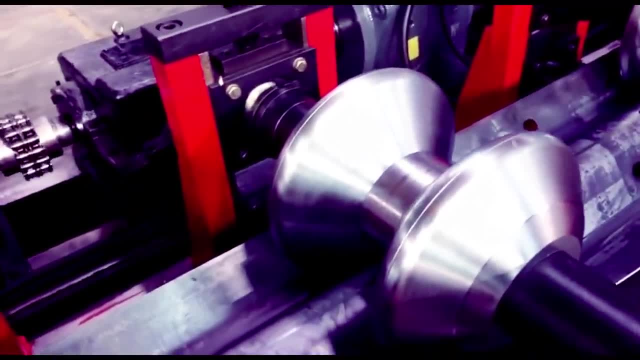 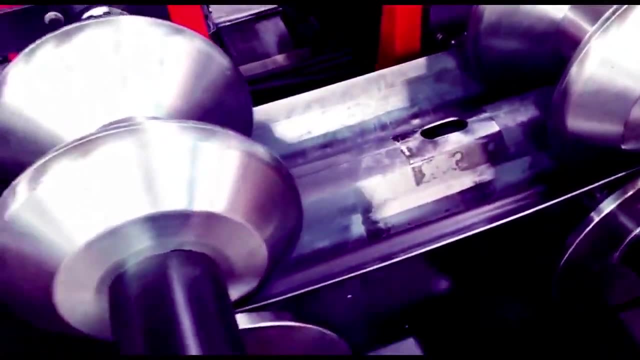 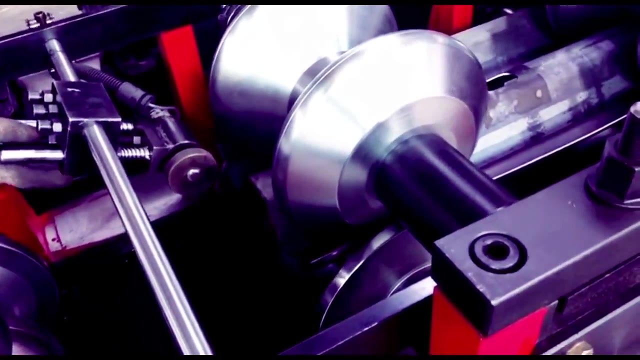 that can help make it more of an even eye-to-eye kind of a thing. Roll forming generally is a longer setup time. When you figure that the average roll form is 12 to 14 passes, you're going to have a fair amount of time setting it up. 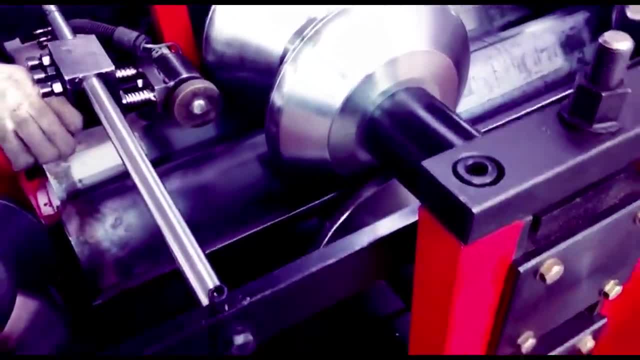 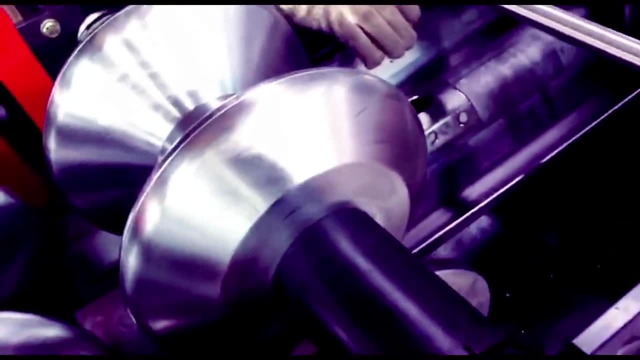 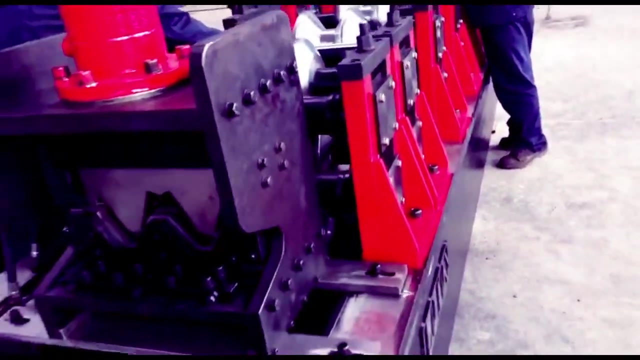 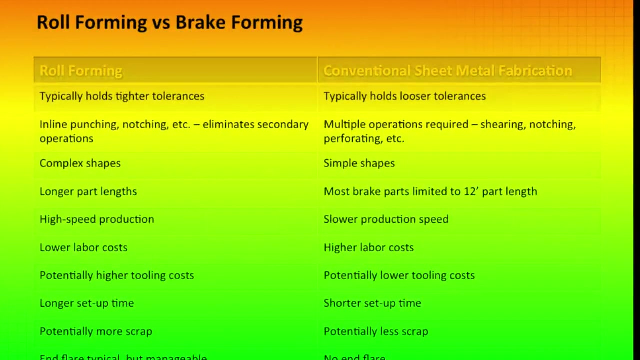 and perfecting the setup before you're ready to turn on and make production. So in that case typically conventional sheet metal fab might have a slightly better advantage there. Potentially more scrap with roll forming versus break forming et cetera. again, amortizing it over a large volume of product makes a difference there. 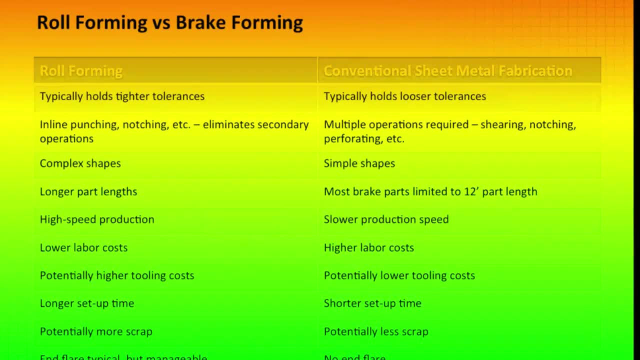 So that's only a potential difference. End flare, which is something we hadn't discussed up to this point, is pretty typical in roll form products And basically what that is is where the end of the channel, the end of the product being roll formed, will flare out. 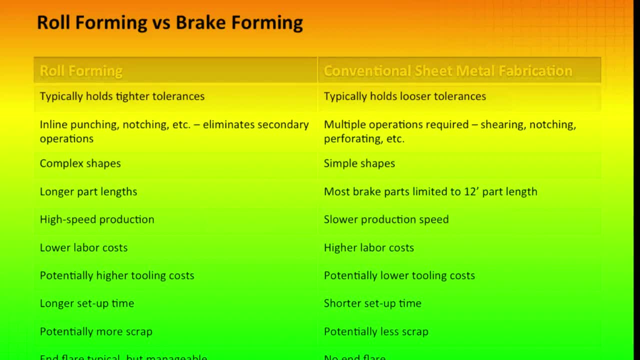 especially at the tail end of the part, sometimes at both ends. You typically don't see that in a break form, product Roll form. you almost always see that. So at least on the surface that appears to be an advantage to break forming. 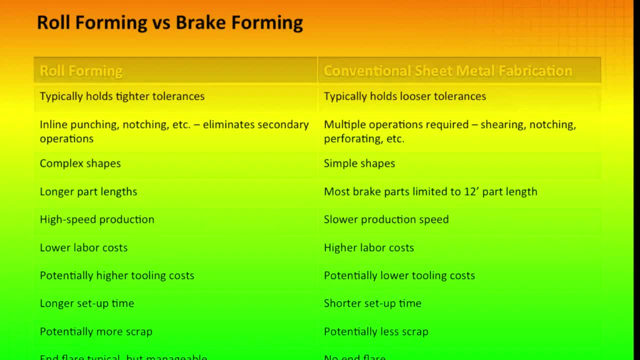 However, there are cases where having some end flare in the roll form product is actually an advantage. We have some customers that use roll form products to stiffen vinyl And having the end flare means when they put that stiffener inside it, it seats itself. 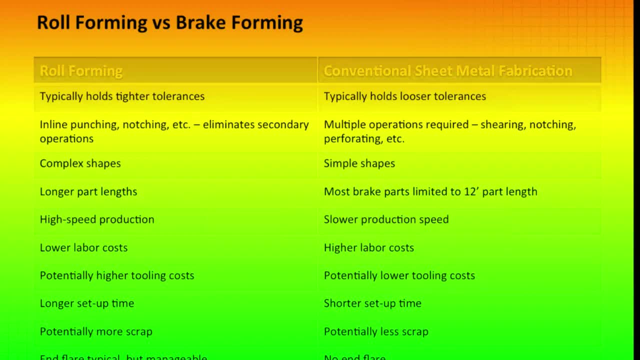 It stays in. It's not sliding in and out of the vinyl product, So they look at that as an advantage. We have some other customers that can't tolerate end flare. Well, we do what we can in the line to minimize it with some over bending. 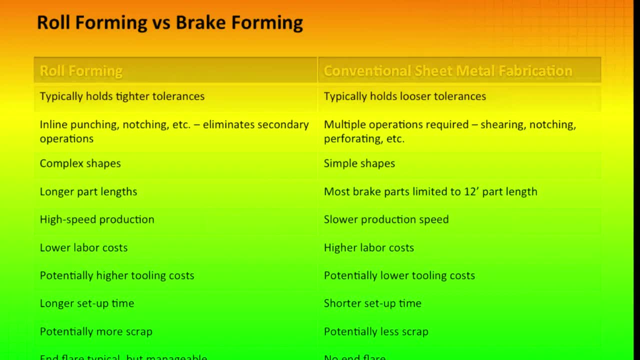 et cetera, special fixtures, And then we have some customers that just it's like no end flare. Well, in that case there are ways to deal with it. as a secondary offline operation, We can deal with it. It's the kind of thing we should talk about. 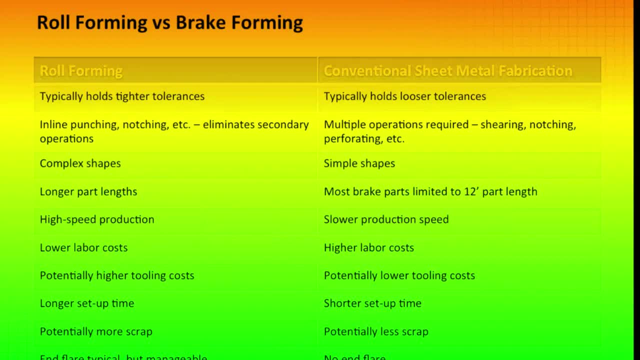 If you have products that are sensitive to that, then we need to know that up front. It will certainly help you as much as we can to deal with end flare. That is a pretty good summary of what we've talked to so far- the pros and cons of the two processes. 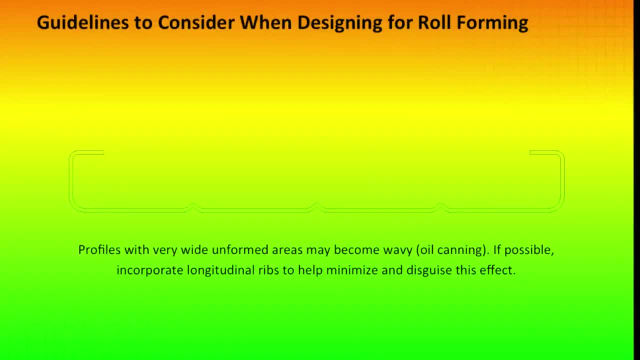 roll forming versus conventional metal fabrication. We're going to go on now, Alan, to the next section here: guidelines to consider. These are some things that if you're designing a product and looking to have it roll formed, or perhaps you've got an existing product and you want to convert it to. 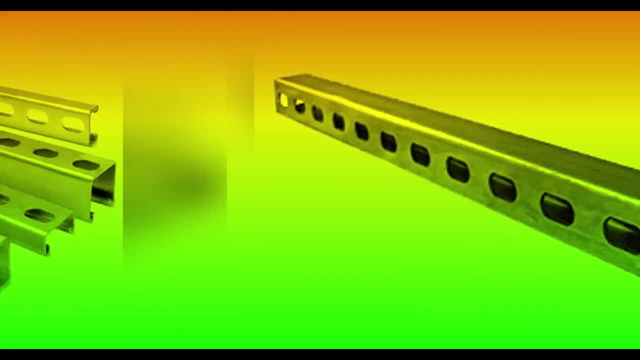 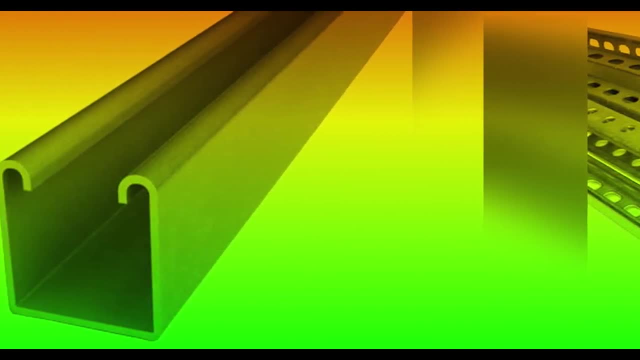 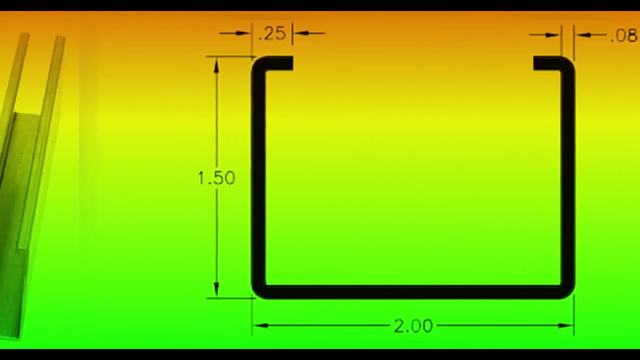 roll form, to take advantage of the efficiencies of the process, reduce cost. these are some things you should take into account. Now. they really are only rules of thumb. They're only guidelines, not hard fast rules- Pretty much everything that we're going to discuss over these next several. 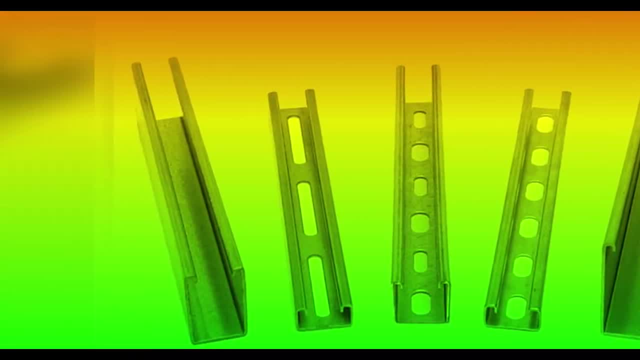 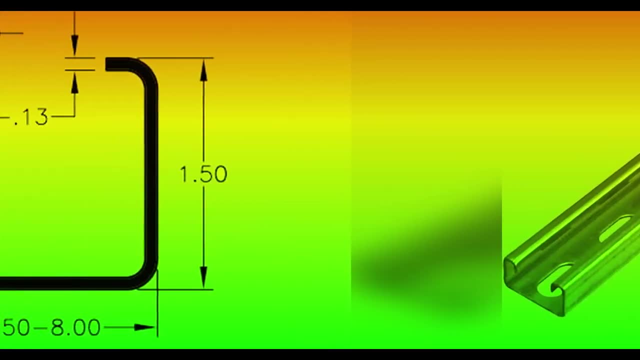 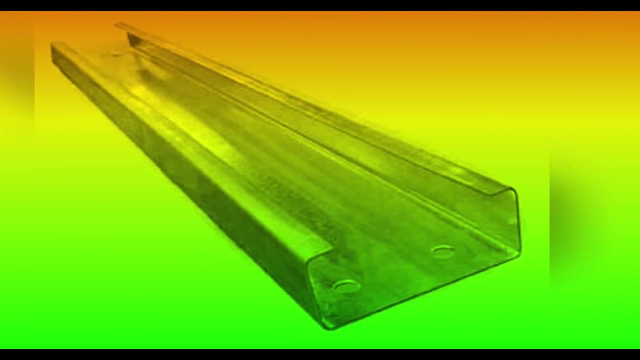 pages. there are exceptions to them, And many exceptions. So all we're saying is: take these things into account and, where you can design around these guidelines, you're going to be benefited when it comes to roll forming your product. So let's take a look at the first one. 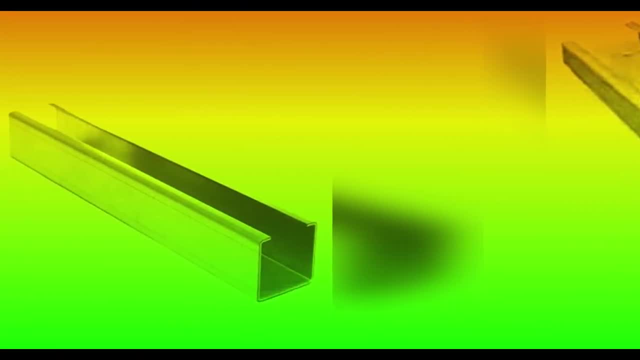 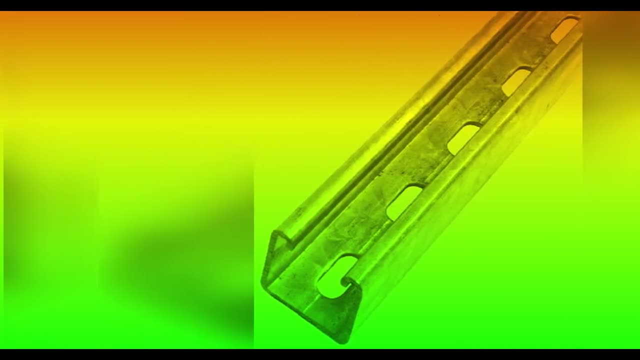 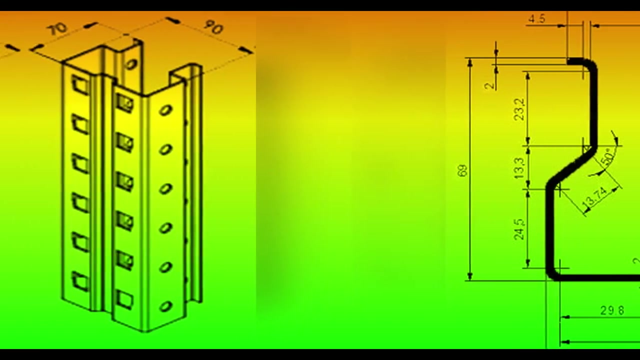 This is a wide panel. This is a wide panel- what you might think of as like a roofing panel, Metal roofs. you see those quite frequently on residential and commercial buildings these days. I saw a metal roof on a building yesterday when I was out walking around. 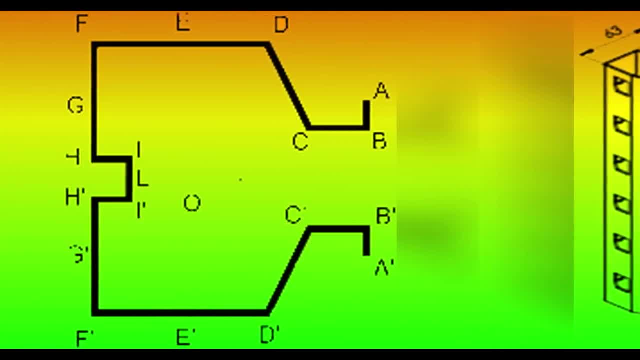 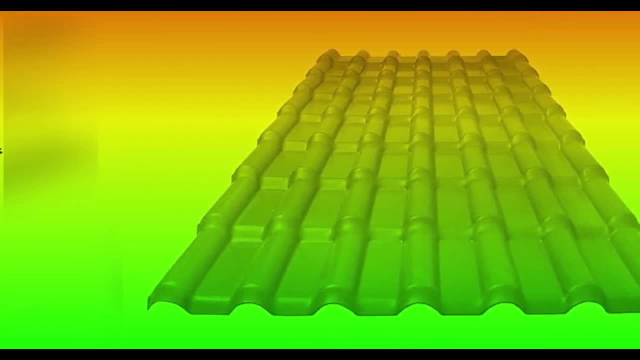 the local community college. It's a metal roof and what I saw when I looked up it was waviness or oil canning. it's commonly called up the center of each of those metal panels. That's very common with wide panels. 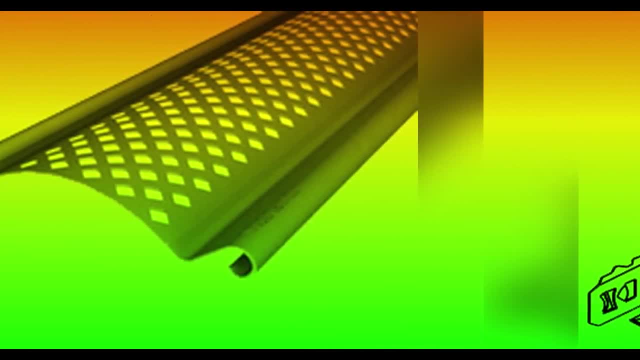 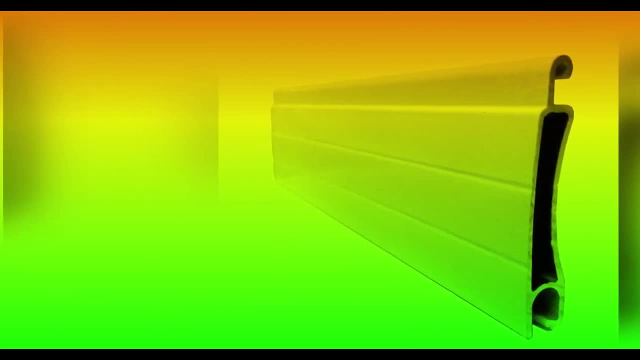 You get much over five or six inches, and especially in the lighter gauge stuff the center is going to wave. So what you try to do is: one suggestion here is add these longitudinal ribs which we've illustrated in this cross-section drawing. 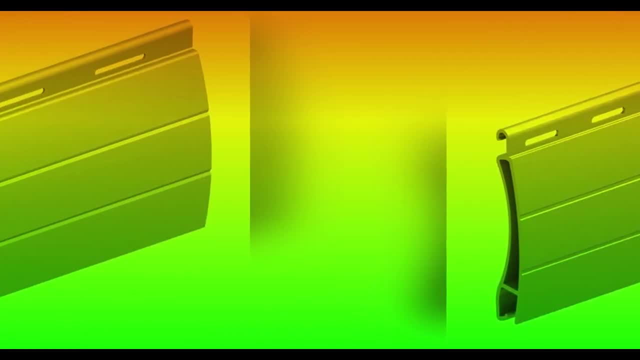 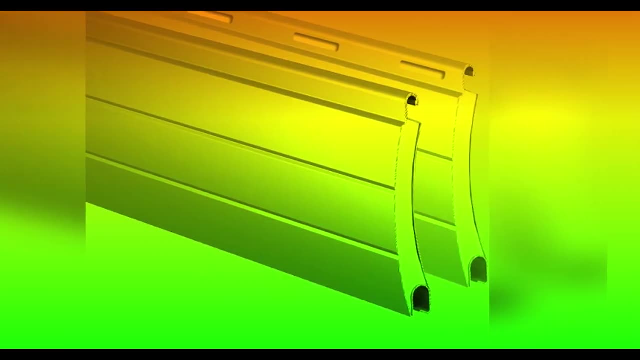 That can help to minimize or at least disguise some of the waviness that's in the center of the part. Other products- you might see that on here- other than roofing panels, building panels, door panels, garage door panels, that kind of thing. 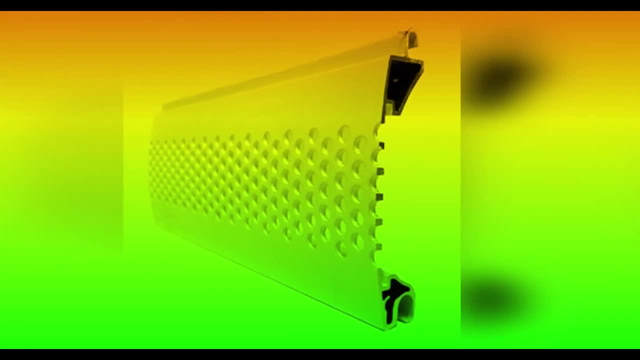 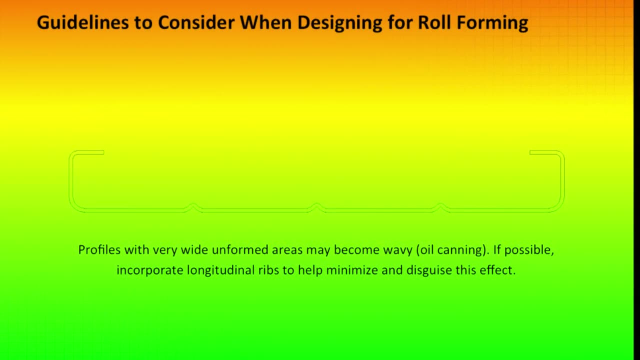 Anything where you've got a wide web light gauge especially, and you're doing forming only on the edges. So one way to compensate for that is with these longitudinal ribs, if that is an issue that you're concerned about. And again, as you get into the heavier materials. 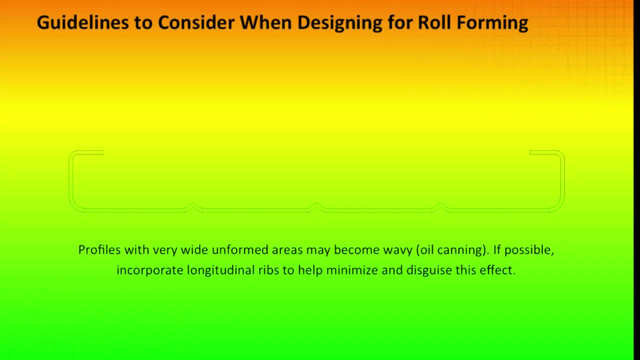 that will not be as visible. The lighter gauge materials- say you know, 22 gauge, 24 gauge, 26 gauge- you're more apt to see some of that oil canning- Versus the heavier, say 14,, 12 or 14 gauge. 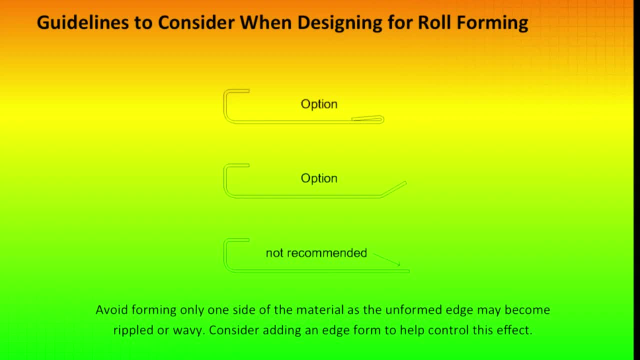 Okay, that's right Now. let's go over to our next page. here, What we're showing in this illustration is a J channel. It could be a cap for a molding or a panel. Quite often all the forming on this type of product is done only on one edge of the stock. 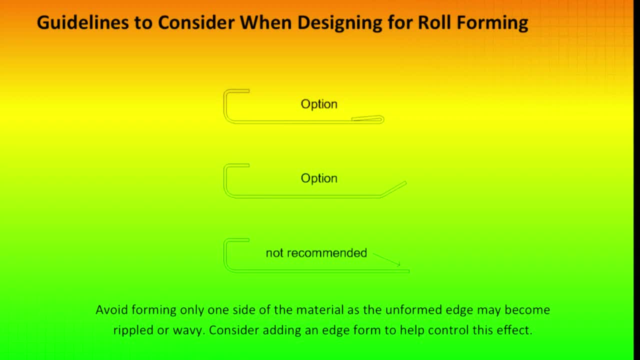 and the other side is left unformed. Depending on your use, you may see the unformed edge get some waviness or some buckling to it If we can add a safety edge, a little hem or even a slight bend to that. 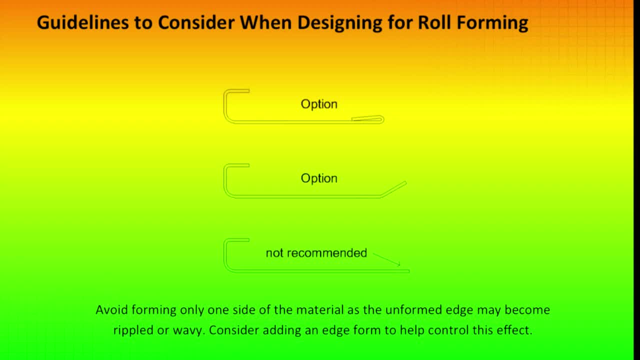 it tends to take care of that waviness along that edge. Now, as I was starting to say, depending on your usage, maybe it matters, maybe it doesn't. If that unformed edge is hidden in the final installation or assembly, then perhaps it's nothing to worry about. 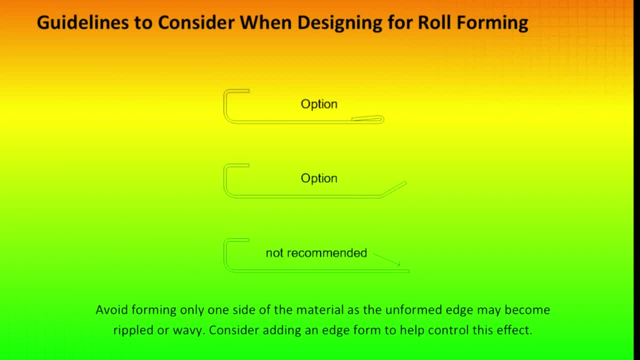 J channels are roll-formed all the time. However, if it shows, then perhaps at least consider putting a slight form on the edge where, at least in the bottom illustration there, we said: not recommended. Well, we'd like to see you try something similar to either of the options shown up above there. 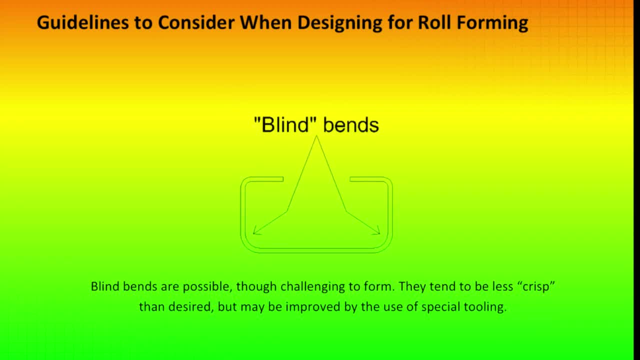 Our next page. we're showing basically an N channel. We're showing basically an N view, a cross-section of a little box channel, And the arrows point into the bottom bends. here We'll call them blind bends And what can happen is those bends. it's exaggerated here in this drawing. 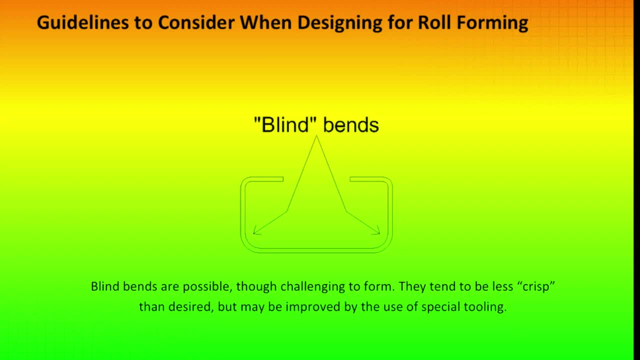 but they can actually become a little less crisp or softer bends than what are formed at the top of this part. There are ways to work around this. If we know that the bottom bends are critical and they need to be very crisp or square, there are things we can do in the tooling to make that happen. 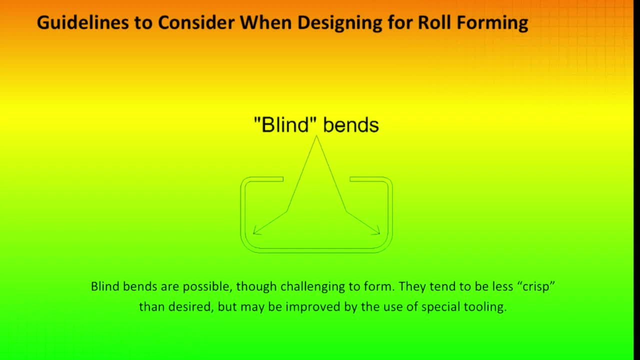 On the other hand, if it's not important to you say, this is just perhaps a stiffening product and it's hidden from view, maybe those larger radii don't matter in your particular use. If they do, though, be sure to call that out so that we can make some provision for that. 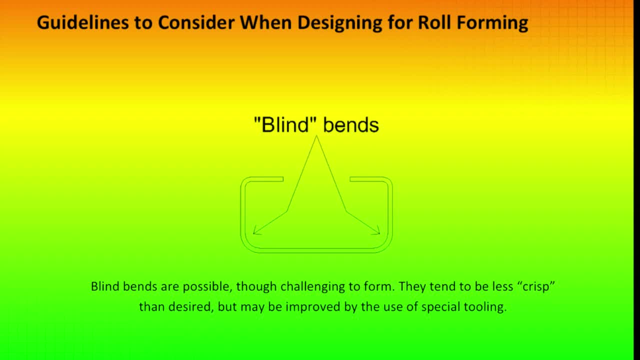 All that happens there is at the point where the top bends cover the bottom bends, so that you no longer have access with the male tool directly with the inside of the bend, and they tend to round to get soft. Again, it depends on your application whether this is a big deal to you or not. 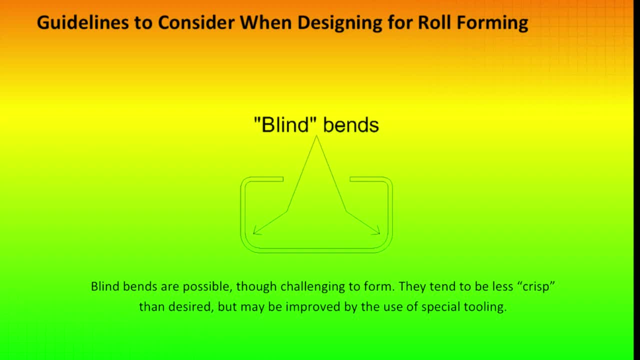 The prime thing here is: just let the roll former know that that's going to be either something you care about or something that really doesn't affect the final use of your product. That's a good discussion to have. Let's move over to our next page, Alan. 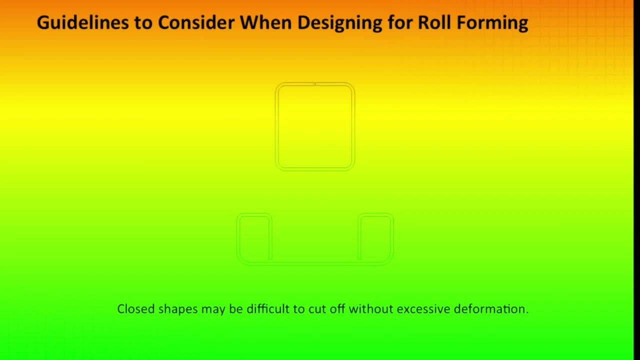 You'll see here a couple of different variations on a theme: closed channels. On the top is a rectangular square tube with an open or a butt seam, and the lower one is basically just a variation of that, where we end up with two rectangular tubes. 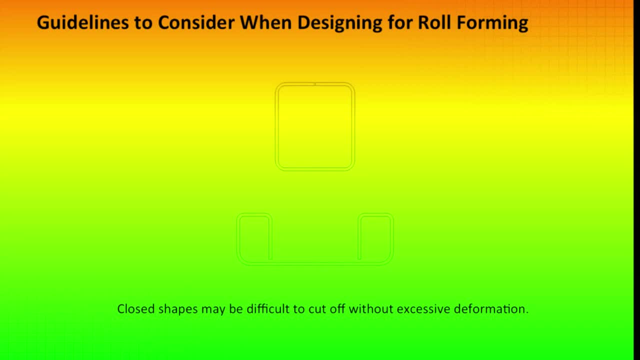 at the extreme left and right of this roll form section Now, when we looked at our slugless cutoff- the servo-controlled slugless cutoff- earlier in this presentation, that's a nice open shape and we can put a set of crop-off shear, slugless, whatever you want to call it. 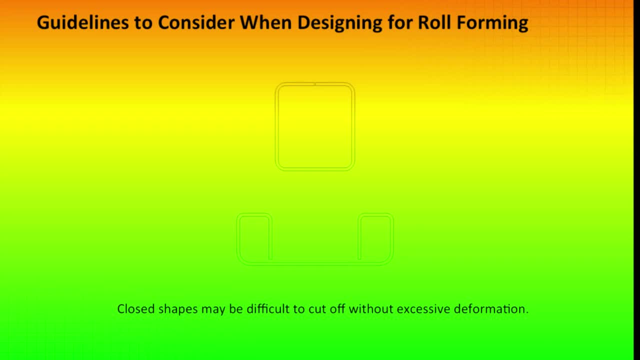 onto these plaits and it can be put into use to cut those products off. This product, either one of these would not lend itself to that because there's a hollow area that we can't get any tooling to support our cut. 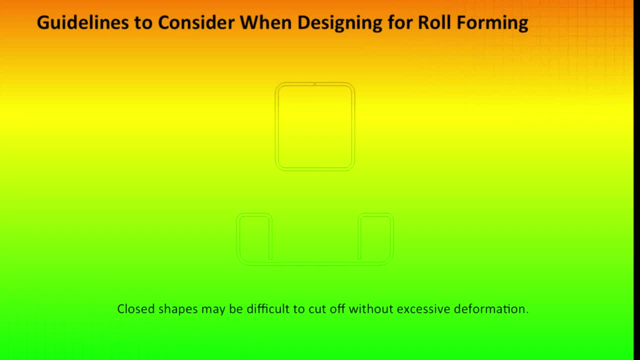 And what will typically happen is there will be some deformation from the cutoff, especially when the blade enters the part. Imagine a blade coming down into the seam of that top square channel and it's going to deform the top until it starts to make the cut. 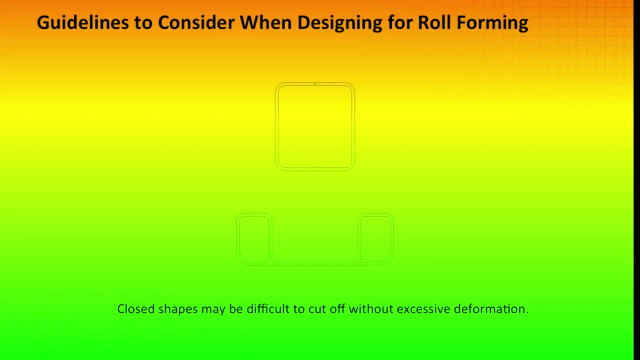 And something similar with the bottom one there as well, The one at the top. we actually have a customer. we make this product for all the time And they're running, or we're running for them, 20-foot lengths which they re-cut by saw so they can cut off the part that is damaged beyond their use. 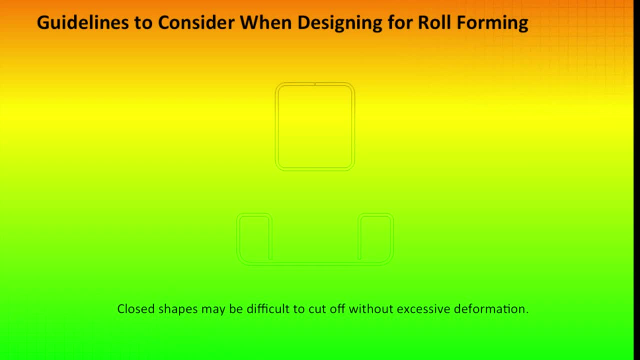 They just take that into account, that there's going to be some of this product that they can't use because of the crushing of the end when it's cut. We have some other customers that actually use it the way it is. Again, it's a hidden part. 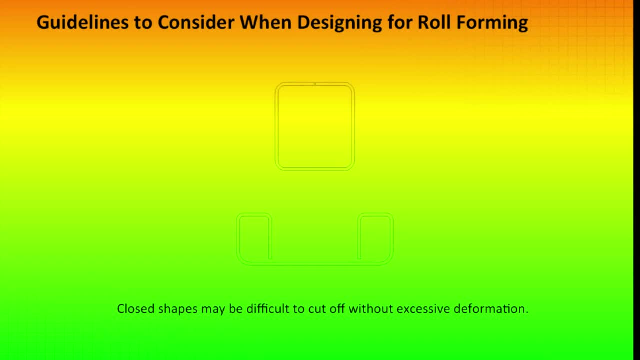 It goes inside something else, Nobody sees that the end is crushed. It doesn't affect the function of it. That's just something to take into account. We can certainly cut off sections like this, but I just expect to see some deformation, a bit of collapse on the tube areas. 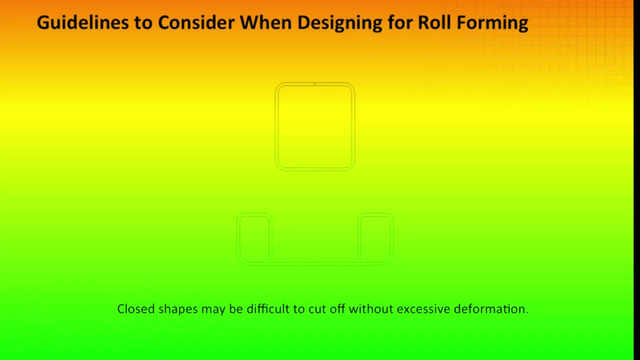 If there's a possibility of adding that gap, having that gap a little bit larger, that would be. That would be a lot better, because then we can get a mandrel in there and hold that and cut that off pretty square for you. So that's one thing to also think about in your design. 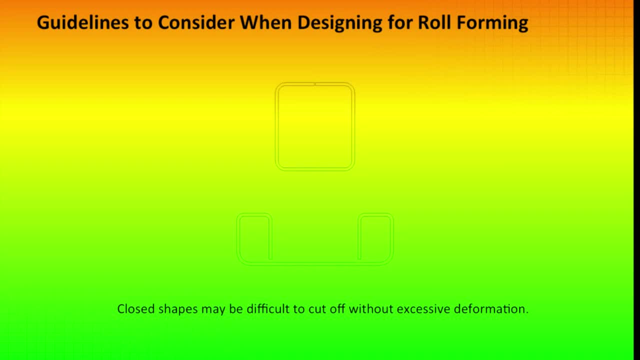 Yeah, we just. you know, each product has to be addressed individually. as to the cutoff method being used, Just keep that in mind and we'll certainly work with you on any designs you have where you think that maybe you can get away with it, maybe you can't. 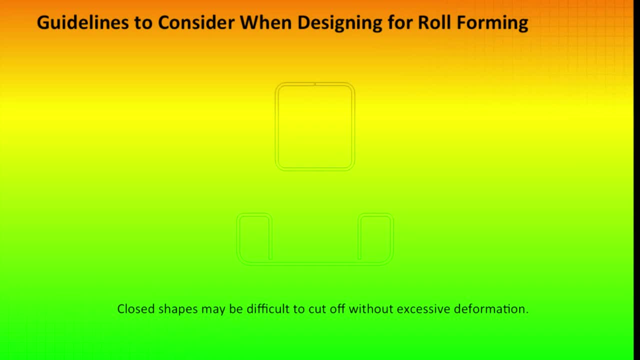 We'll be happy to give you some guidance. Cutoff is a big issue when it comes to roll forming, so we'd like to get in early and help you work through those issues in the design stage, if at all possible. Our next page: here we see a nice open section, kind of the opposite of what we just talked about in the last shot. 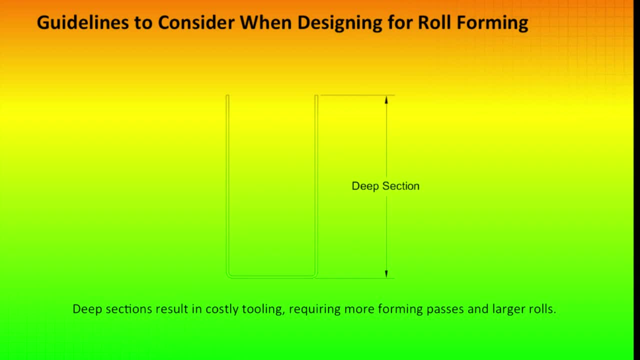 Nice deep U-channel, which certainly is a roll formable product. What you get into here as the section gets deeper, you also get into higher tooling cost, And imagine a wide strip of material that would be required to make this channel. If this is 6 inches deep and 2 inches wide, you're looking at approximately a 14-inch wide strip. 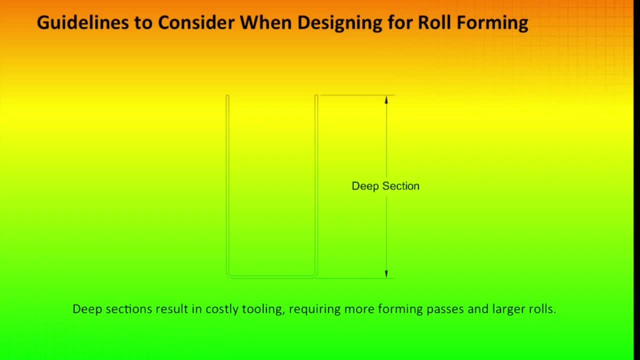 Well, you've got to have roll tools that cover that and start the bends, and it takes more passes to finish these long legs than it would if the channel were shorter. So, generally speaking, the deeper the product, the more expensive tooling gets. 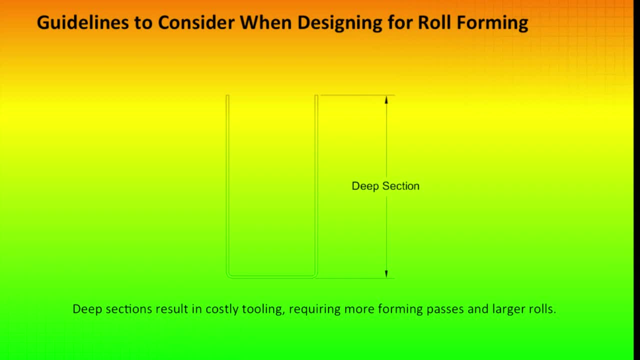 Sometimes you just don't know. You don't really have a whole lot of choice. You need a deep channel, you need a deep channel, But many custom roll forms are not going to have necessarily a set of roll tools that will go indefinitely deep. 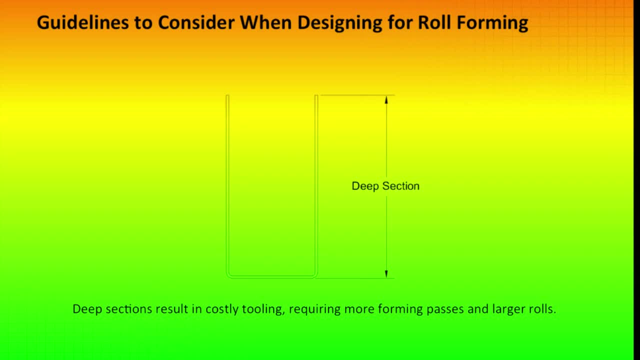 Here at Roll Form of Jamestown we generally limit ours to 3, 1⁄2, perhaps 4 inches because of the mills that we have here, So you're also limiting your options on what existing universal channel dies may be available. 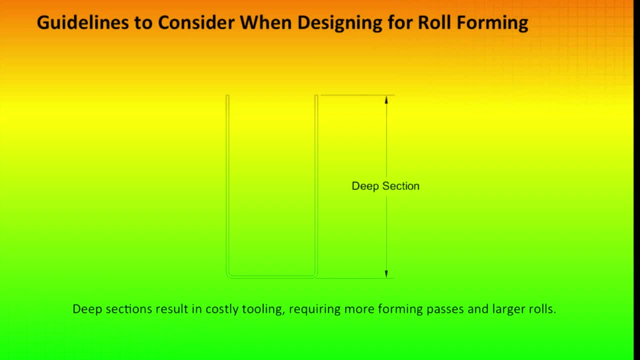 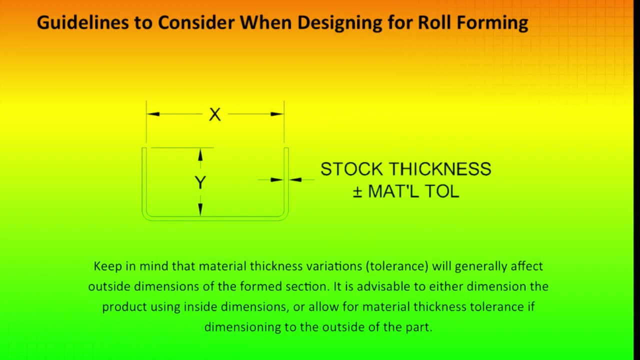 Now all that said, Can this be roll formed? Yes, And it is. every day Just deeper means more expensive from a tooling standpoint. Next page here Just some things to keep in mind when it comes to tolerancing your drawing. 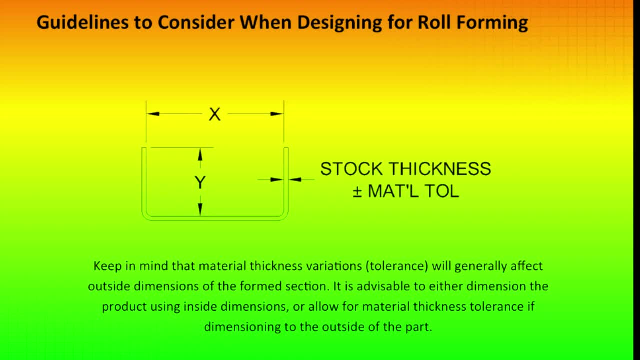 Like any fabrication process, roll forming works with coiled material or blanks in some cases, But we still have the material thickness tolerance to take into account. Typically, what happens is roll forming forms the metal. They're not as flexible around the male tool, which is the inside of the part. 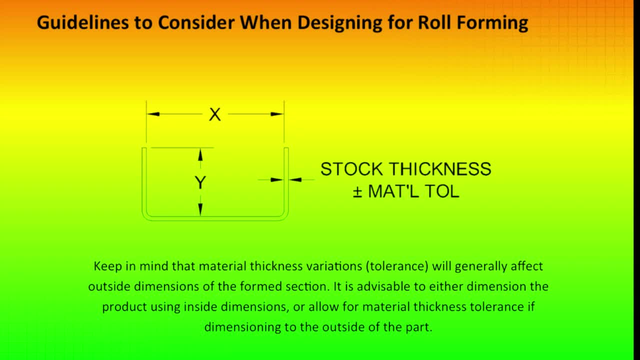 And so inside dimensions are actually more consistent, whereas the material thickness variation shows up on the outside of the part. If you can, and it's practical, to dimension to the inside of your channel, you'll find that the variation is much less than measuring to the outside. 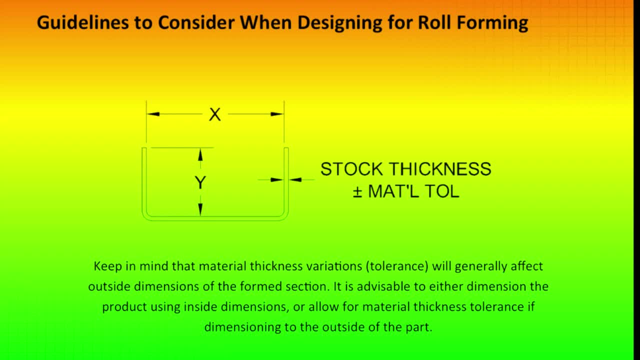 Now, having said that, There are things we can do If it's an outside dimension, If it's not as difficult to you, we can put control passes in there to control, let's say, the width of this channel, regardless of the material thickness variation. 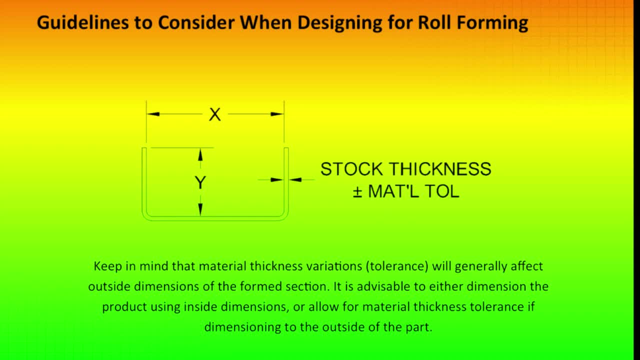 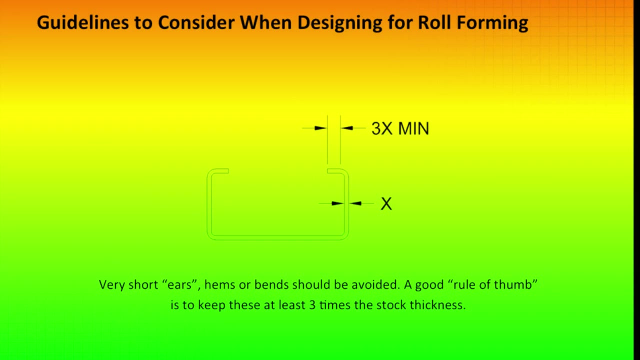 We just need to know that upfront and have the part toleranced appropriately so that the tools and the process meet your needs. Next page here: This is one that's pretty important when it comes to roll forming. Quite often You'll see a C channel. 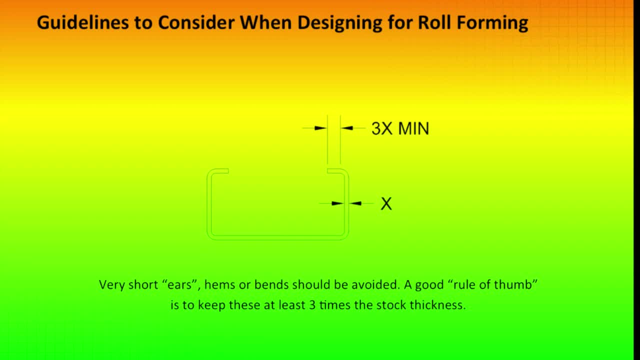 Or a little box and some short returns, or ears as we often call them. There's kind of a limit there If you, if you, can maintain a minimum of three times material thickness as the dimension for the straight segment of the year makes a formable part. if it goes to less than that becomes very difficult to form and especially as the material thickness increases. 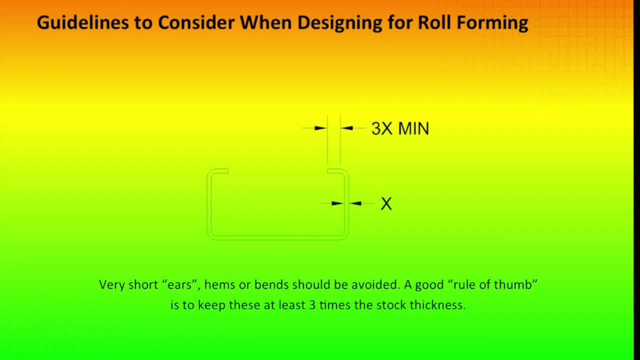 Just imagine that you're actually using An effect, a lever to make that bend in the roles And there's just not enough to make the bend. It won't grab it and and make it form crisply and evenly. Sometimes it'll even damage tooling if it's heavy gauge or high strength, and that the bends are just too short. 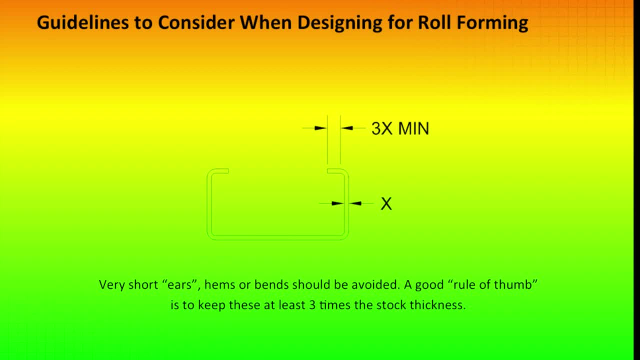 So here's the rule of thumb: Three times material thickness as a minimum On the straight segment of any returns. Even if it's, even if we can make it with bend, with less than that real hard on tool, It's going to shorten their life and it'd be a great deal of tool maintenance and repair that runs into some money. 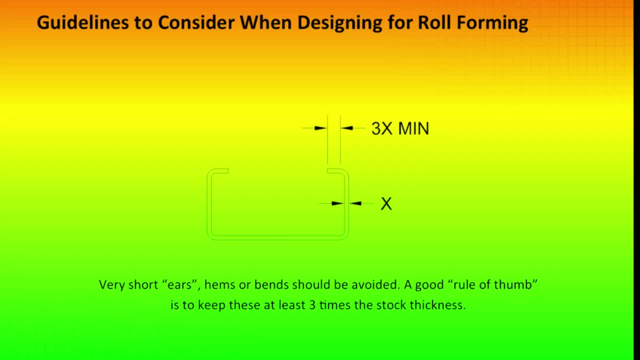 So, and of course, as it wears, it's harder to maintain the integrity of the power. All right, Next page, please, Ellen. Here you should see a roll formed part with a very large arc or radius. These are surprisingly difficult to control. 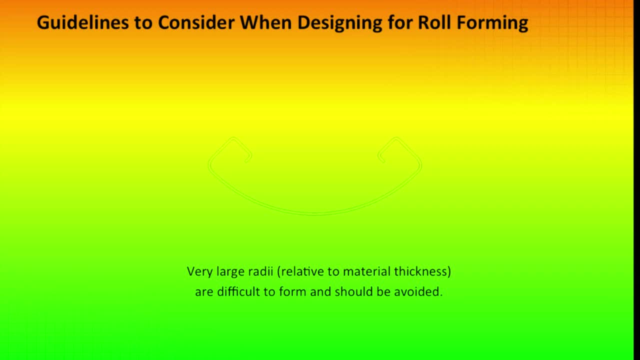 Because the radius is so large, and especially in relationship to the material, It's really hard to get the bend, the arc to set and stick. The arc tends to want to open up. I saw a job once where we formed it up very close to what's demonstrated here. 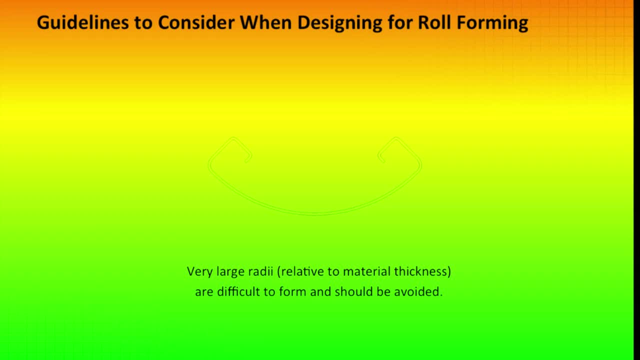 When exit the last pass, the whole thing opened up, So it was nearly flat again. Can it be done? It can be, But quite often what you'll see is, rather than a one single large true radius Or arc, It ends up being a series of shorter bends and lines. 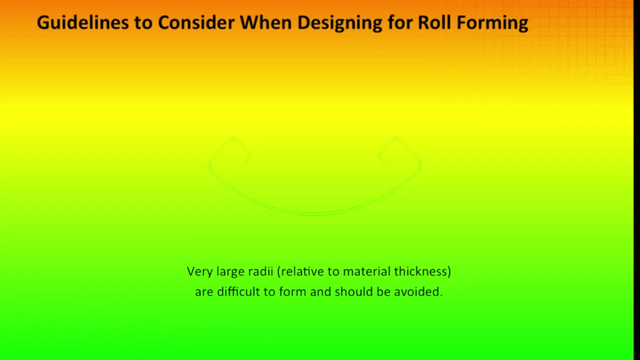 So it's almost like faceted, As opposed to being a true radius or a true arc. It's generally a series of shorter straight bends that will simulate an arc. So if it's high strength material, If it's something with a lot of spring to it, 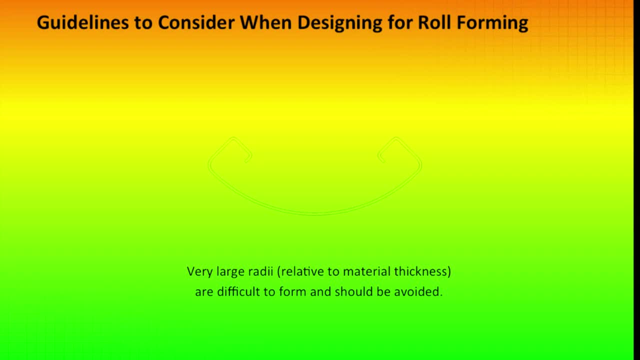 Stainless, Pretty tough to control But it's going to work Pretty tough to do. Just so much over forming root card that it's very difficult to make that Unless it ends up being faceted. Let's go on to our next page. 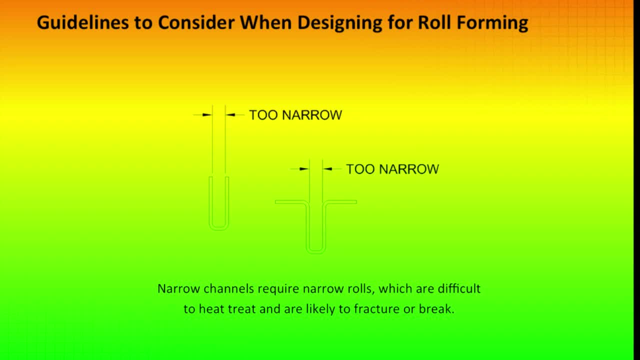 This. we're demonstrating a couple of narrow channels- And you'll see that it's called out there. They're both too narrow. Well, they are certainly producible. We produce some channels here that are much narrower than what's shown in this sketch. 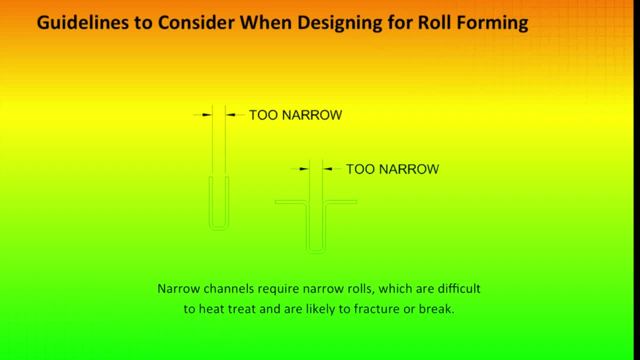 We make one product that's got a 5 16ths opening on the inside With 11 gauge walls. The problem comes is not that you can't make the part. They are certainly roll formable, But it's very hard on tooling. 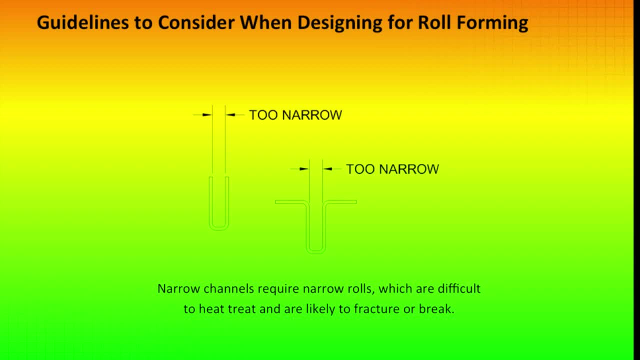 Both in tooling production. If you can imagine, It would have to be quite a narrow slice, A skinny slice of tooling that would have to go down inside these channels To maintain the opening while the part's being formed around it. Well, those tools are challenging. 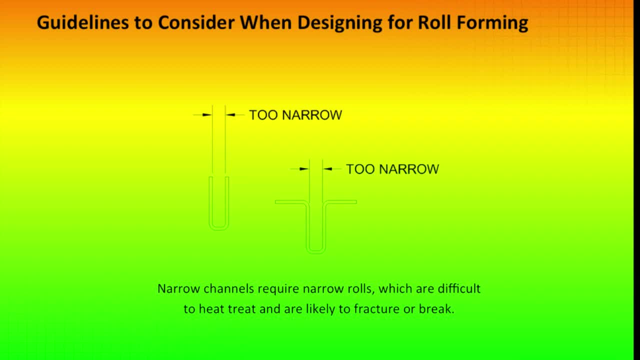 When it comes to heat treating, They like to warp. They're that thin. They're also difficult as you get into the heavier gauges To keep from fracturing or cracking. We do have this one particular job, That that's what happens. 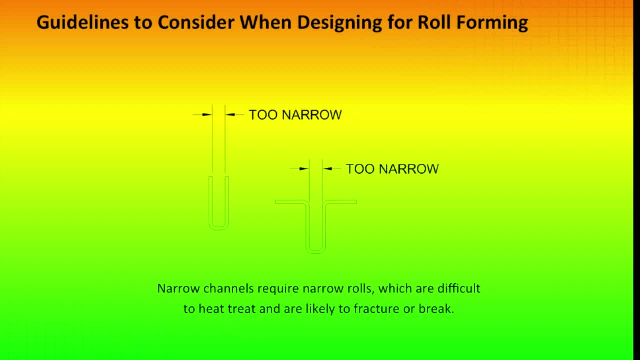 We find that every few runs we have to replace some of those thinner slices Because they fatigue and crack. There's a lot of side pressure, Not much tool still there, And so they crack And it just becomes a consumable part of our production run. 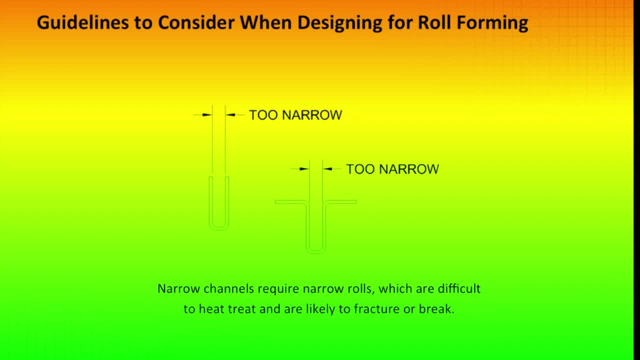 We keep spares on hand. So, very narrow channels: Yes, it can be done. Just be aware that there are some tooling issues involved And it will certainly work with you To work through whether the material gauge, The material properties And the channel width is appropriate. 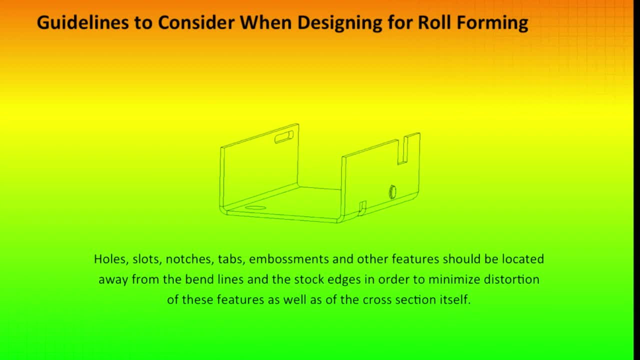 If they all fit together. Our next slide- Actually the last one in this presentation As far as guidelines. We're showing here Kind of a short sample, Kind of a funny looking new channel. Basically, what we've done here Is we've included in the sketch. 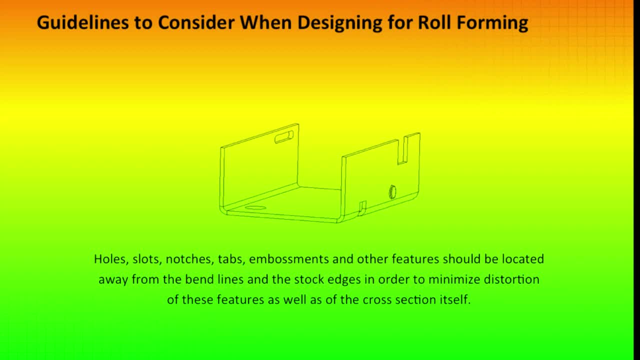 Some features that might be typically seen in a roll form part That's most often pre-punched: The ob round slot at the top Right in the rear of the picture. There's a small round hole in the bottom of web Very close to a bend. 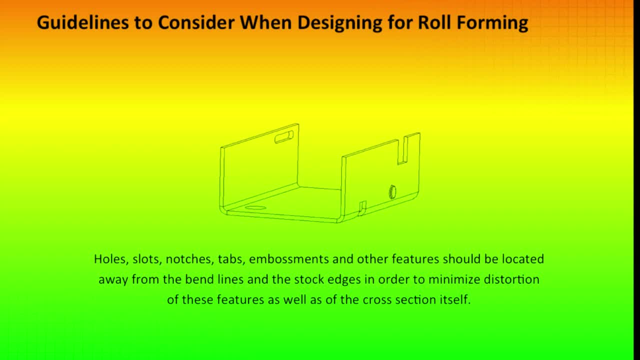 If you examine the right side of that same illustration, There's obviously a notch That goes around the bend. There's another notch that comes in from the edge of the stock Part way down the side, And then between the two of them,